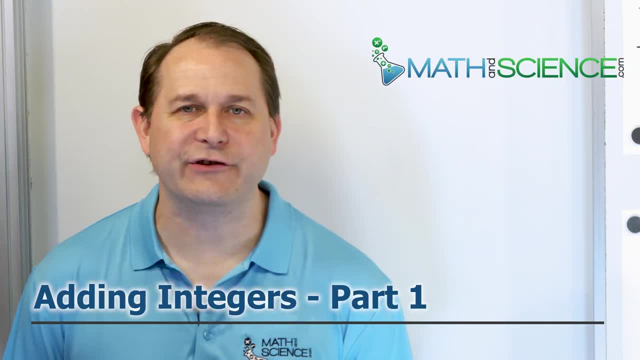 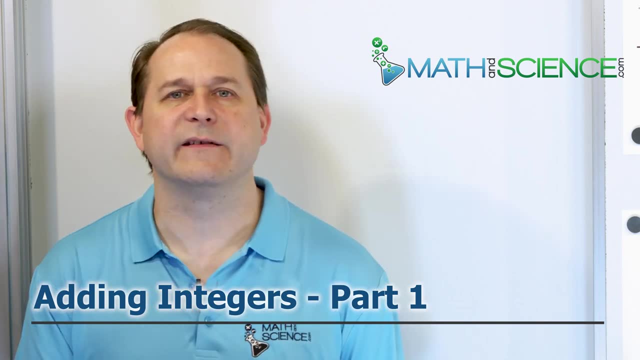 Hello, welcome back. The title of this lesson is called adding integers, which is a fancy way of saying adding negative and positive whole numbers. right, And we've been doing a little bit of that in the last lesson, but here we're going to really conquer all of the cases, So we're going to be 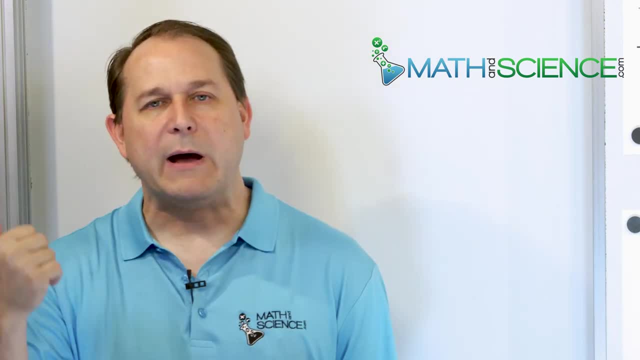 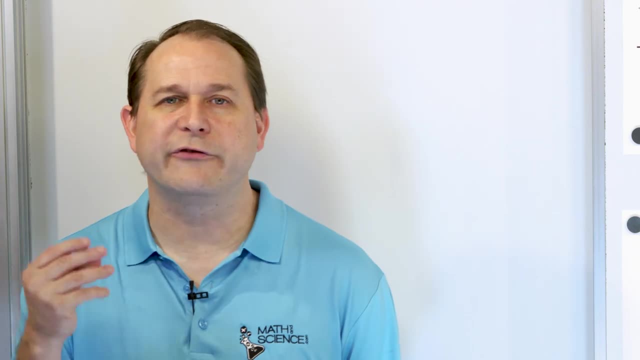 adding a positive number to a positive number, a positive to a negative, a negative to a negative, and so on and so forth. Now it seems complex at first, but I promise you, with practice you will start to get the hang of it and you won't be really having to memorize anything. 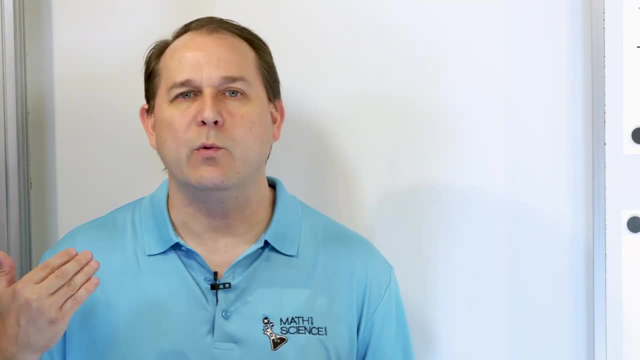 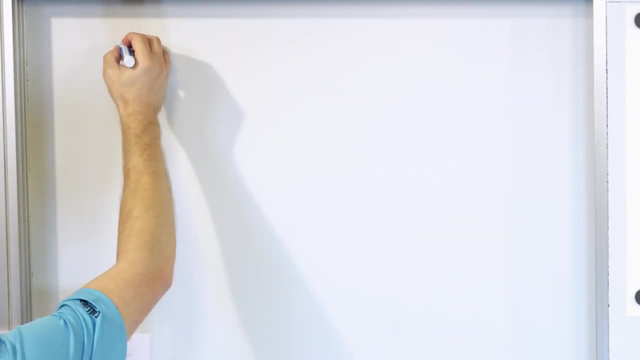 but you will have to practice your skills. Eventually it will become like second nature what we're doing. So let's talk about this. Let's talk about the easiest case that you know about. Let's say that you're adding a positive number. right, That's what this means: positive number. 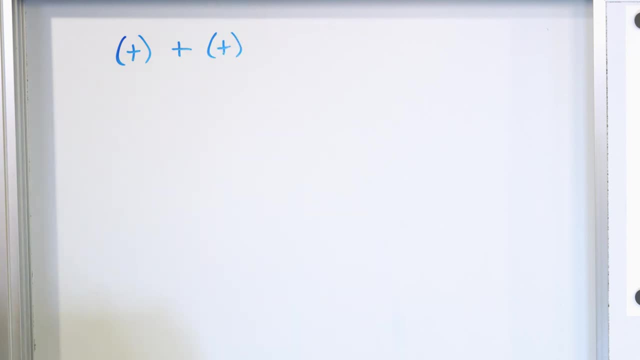 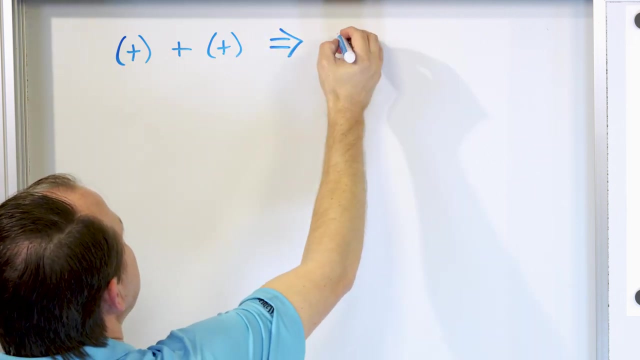 and you're adding to that another positive number, right? So what is going to be the sign of this answer? right, If you have a positive number and you add to it a positive number, you're always going to get a positive number back, And the easiest example I can come up with is just something. 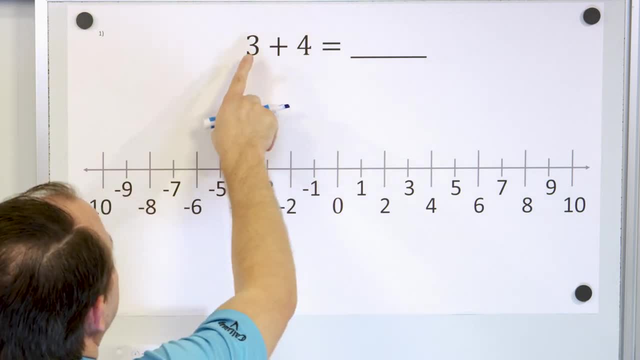 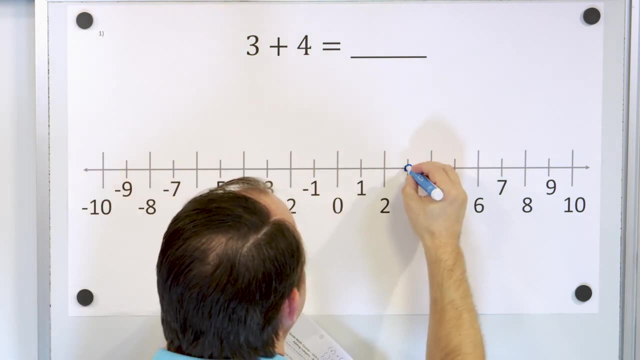 like 3. plus four. What does three plus four mean? It means you start with three dollars and you accumulate or add to it four more dollars. So, on the number line, if you start at the three dollar position, this is your starting position and you add four dollars to it, it means you go to the. 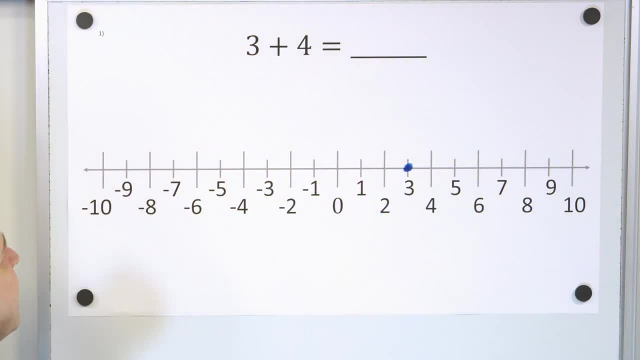 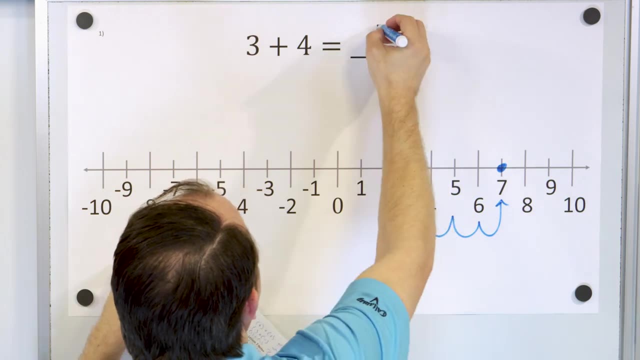 right. So when you add you go to the right and when you subtract you go to the left. So if you go four positions to the right- one, two, three, four- then you land on the number seven and the. 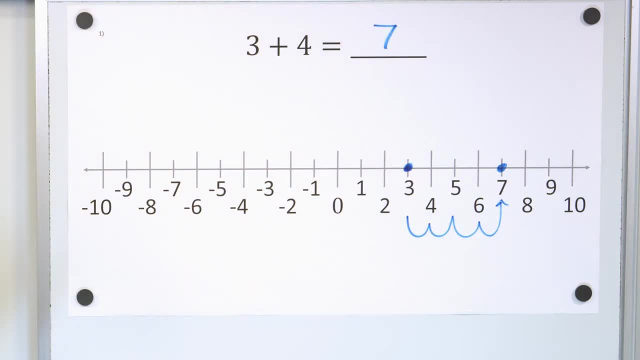 answer we get is seven, All right, and so you then know that three plus four is seven. So easy enough. that's the kind of stuff we learned long, long time ago. Positive plus positive will always give you positive, because if you start with a positive number and you add to it, you're always 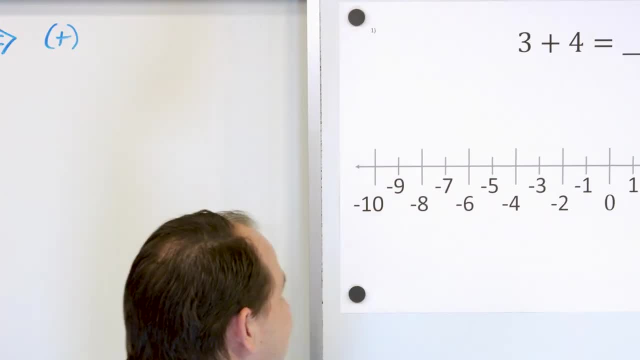 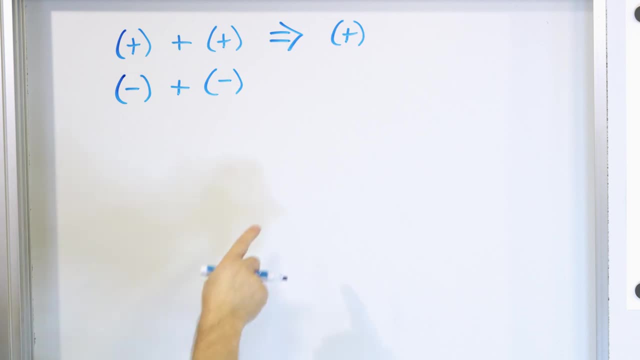 going to get a larger positive number. Now let's think about another case, an equally important case. Let's say you start with a negative number and you add to that another negative number. What are you going to get as an answer? Well, it turns out that if you add a negative number to another, 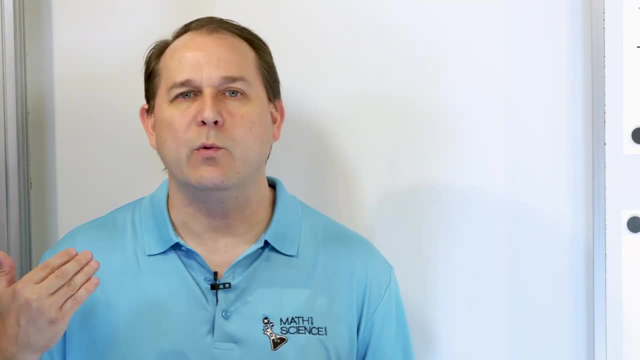 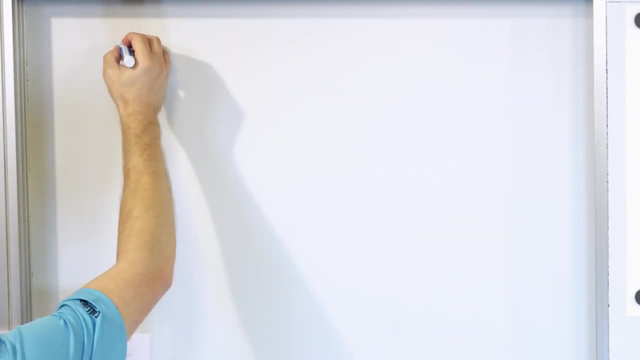 but you will have to practice your skills. Eventually it will become like second nature what we're doing. So let's talk about this. Let's talk about the easiest case that you know about. Let's say that you're adding a positive number. right, That's what this means: positive number. 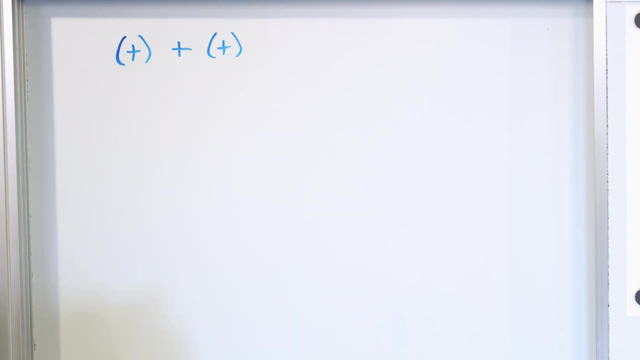 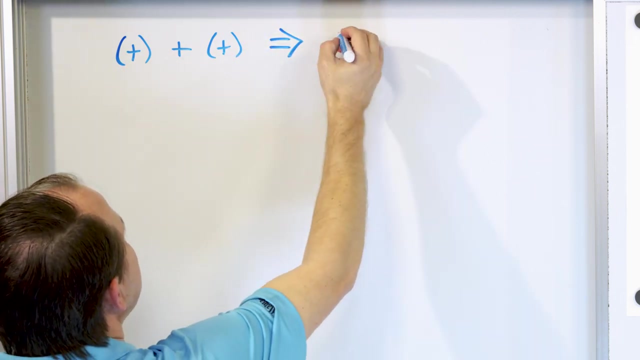 And you're adding to that another positive number, right? So what is going to be the sign of this answer? right, If you have a positive number and you add to it a positive number, you're always going to get a positive number back, And the easiest example I can come up with is just something. 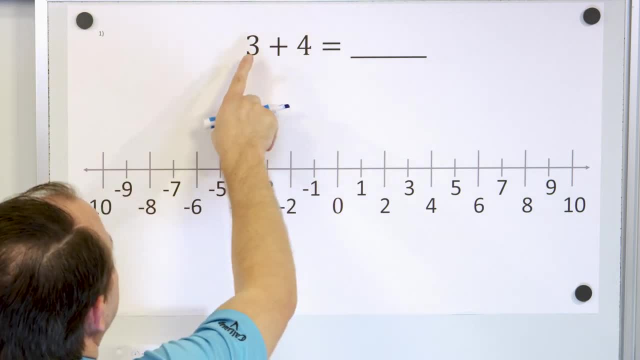 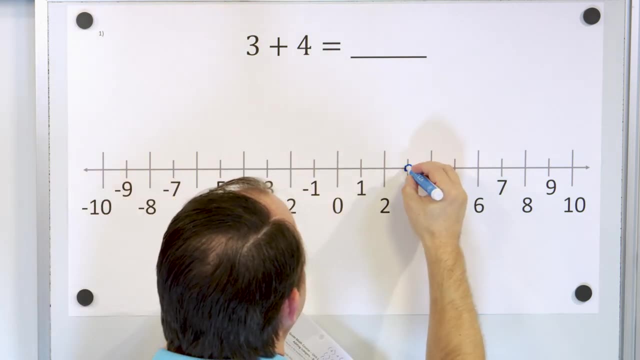 like 3. plus four. What does three plus four mean? It means you start with three dollars and you accumulate or add to it four more dollars. So, on the number line, if you start at the three dollar position, this is your starting position and you add four dollars to it, it means you go to the. 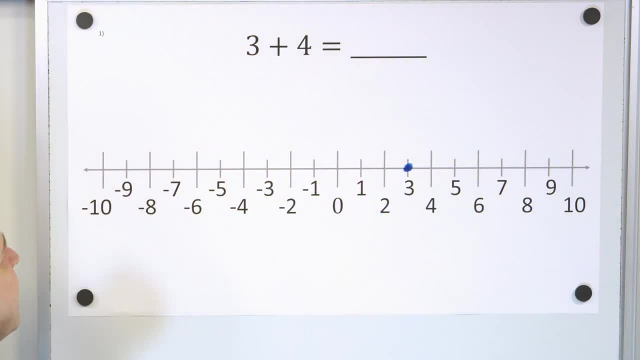 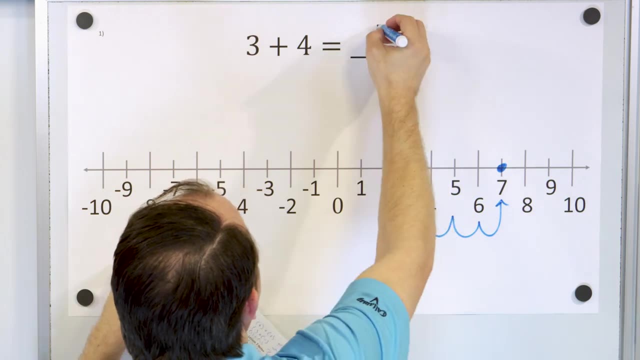 right. So when you add you go to the right and when you subtract you go to the left. So if you go four positions to the right- one, two, three, four- then you land on the number seven and the. 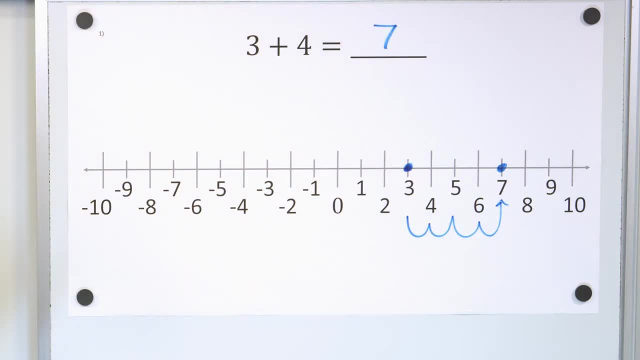 answer we get is seven, All right, and so you then know that three plus four is seven. So easy enough. that's the kind of stuff we learned long, long time ago. Positive plus positive will always give you positive, because if you start with a positive number and you add to it, you're always 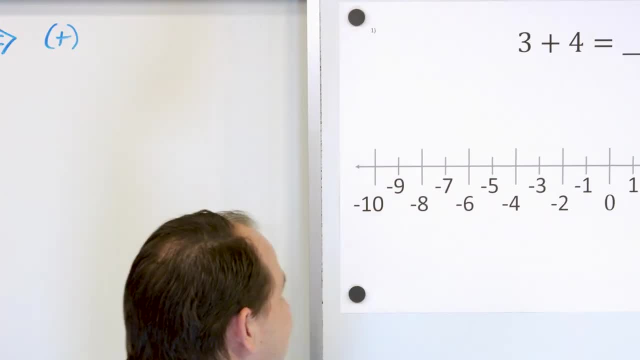 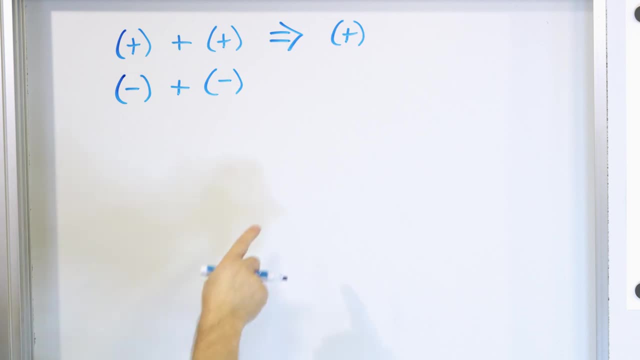 going to get a larger positive number. Now let's think about another case, an equally important case. Let's say you start with a negative number and you add to that another negative number. What are you going to get as an answer? Well, it turns out that if you add a negative number to another, 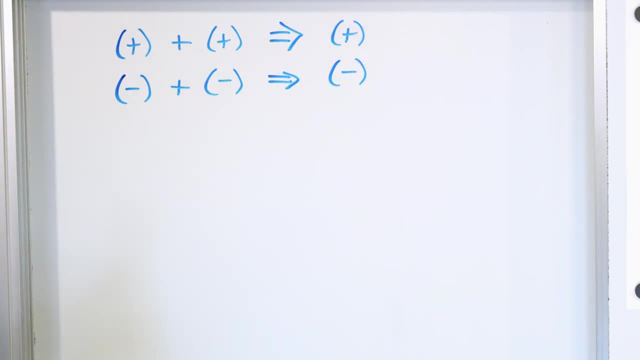 negative number. you will always get as an answer a negative number. Why is that? Because what is a negative number anyway? A negative number is debt. right? That's what negative numbers mean, or one way to think about it. So if I have negative three dollars, then I actually just owe someone three. 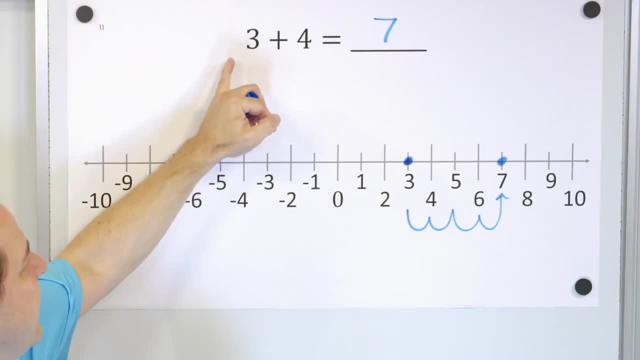 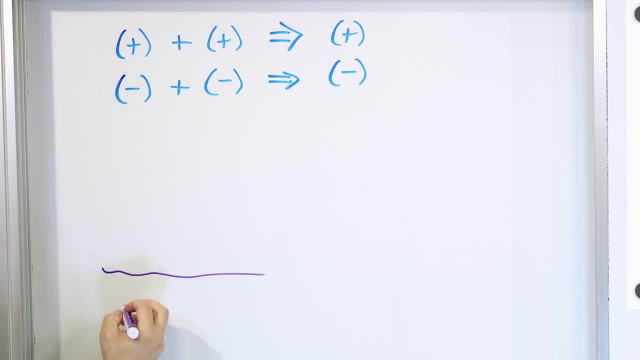 dollars. I don't have that money. I owe someone else that money. So instead of three plus four, let's do a similar problem down below over here. right, Instead of three plus four, we will say negative three and we'll add to that negative four. 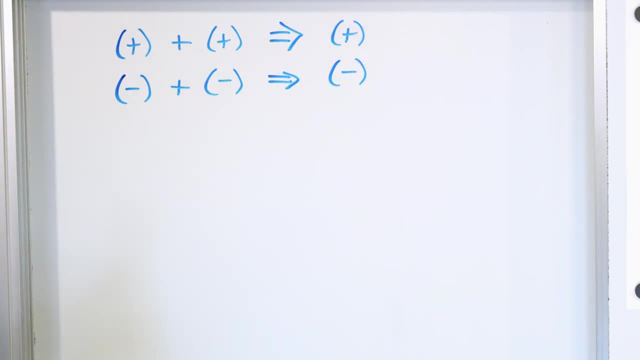 negative number. you will always get as an answer a negative number. Why is that? Because what is a negative number anyway? A negative number is debt. right? That's what negative numbers mean, or one way to think about it. So if I have negative three dollars, then I actually just owe someone three. 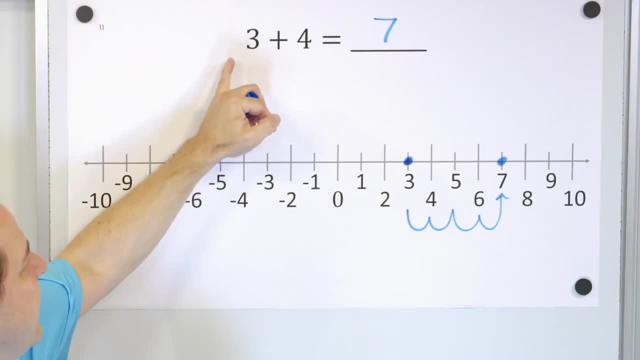 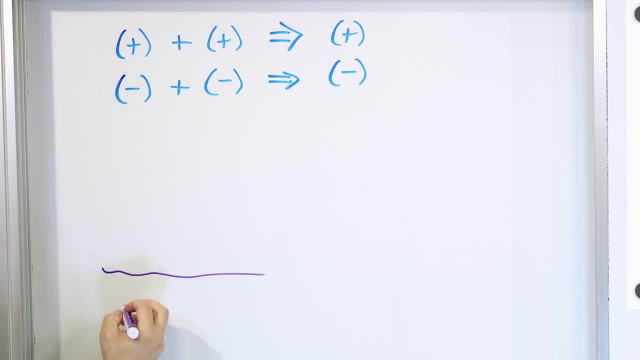 dollars. I don't have that money. I owe someone else that money. So instead of three plus four, let's do a similar problem down below over here. right, Instead of three plus four, we will say negative three and we'll add to that negative four. 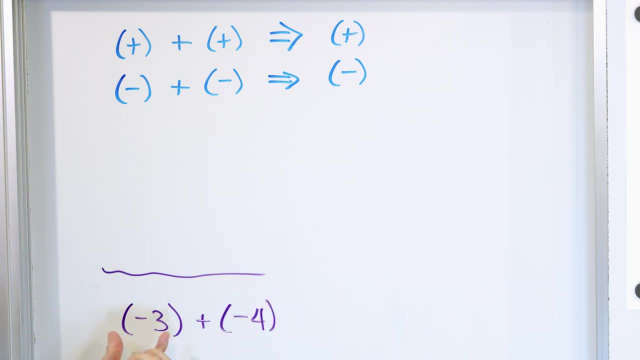 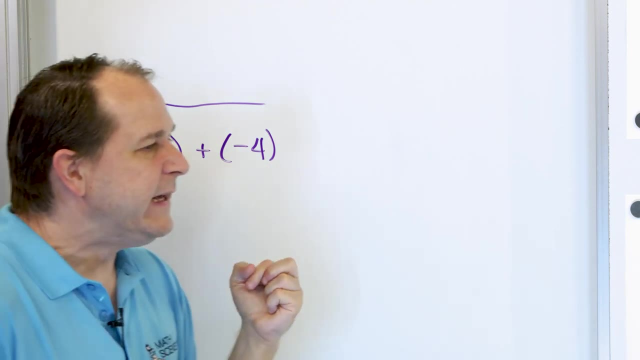 So it's, like I said, a negative plus a negative. So what does this mean? It means I start out by having a debt of three dollars. I owe somebody three dollars, but I add to that more debt, right, So I'm already in the hole because I've already owe somebody three dollars. 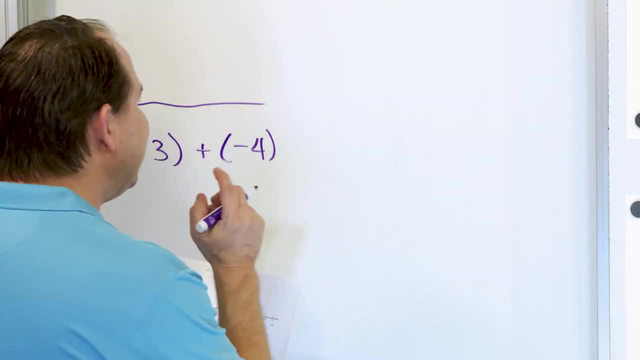 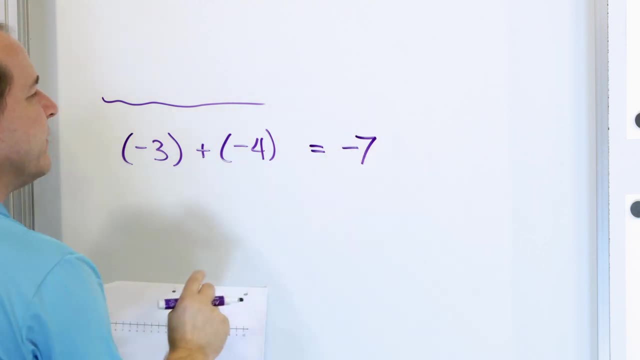 but then I have to go borrow more money for more dollars. So what do you think is going to be the answer? If I already owe three dollars and then I borrow four more dollars, I'm going to have a total debt of seven dollars. So negative plus negative always gives me a negative answer. 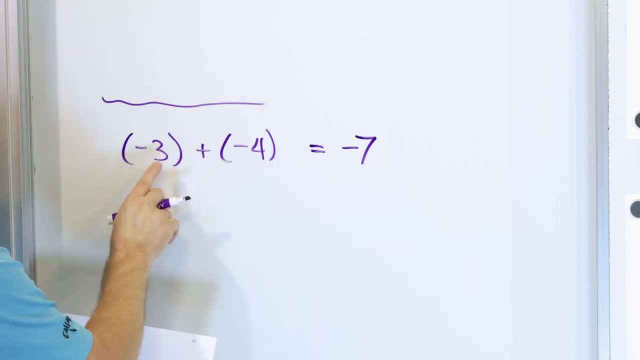 And notice what we did To get the number In our mind. we just took three plus four and made it seven. We still have to add the numbers, but because it's negative plus negative, which is debt plus debt, we kind of add. 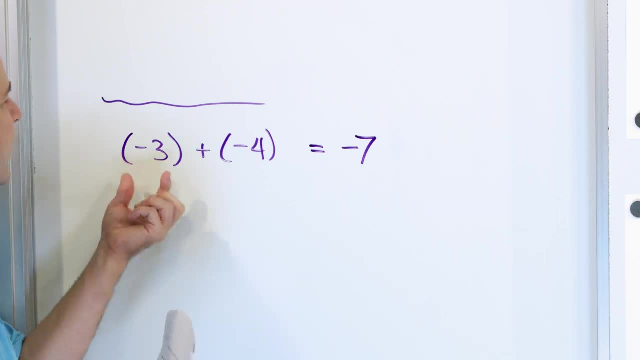 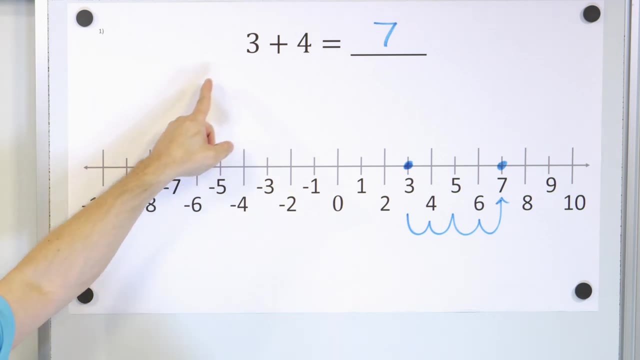 the numbers and then we just stick a negative sign on the front of it. So a negative plus another negative will always be a negative. If we were going to use the number line, then negative three plus negative four would mean that I would start at negative three, but I would be adding to it. 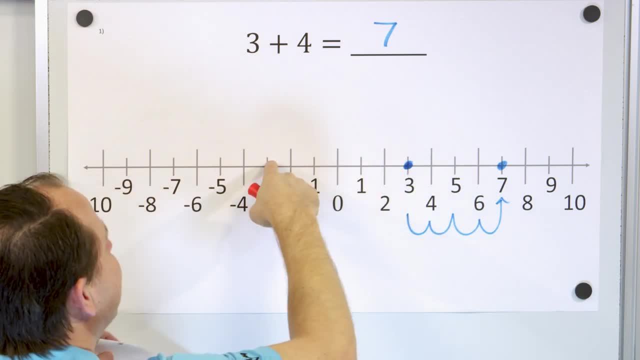 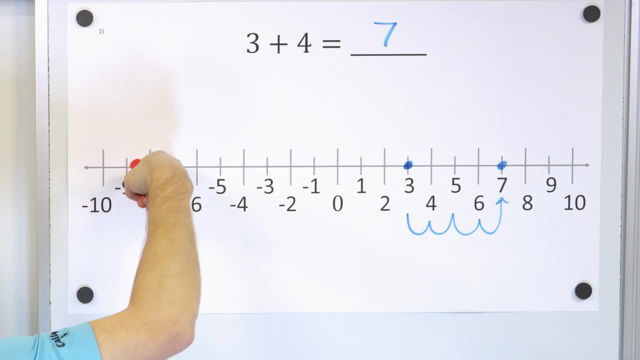 more debt. So I'm not going to go to the right because I'm not getting more money. I'm going to have to go to the left because I'm borrowing four dollars. One position, two position, three position, four positions: I land on negative seven. So, starting with negative three, going one more in. 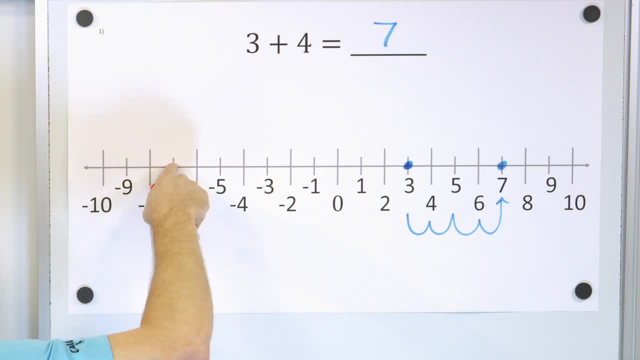 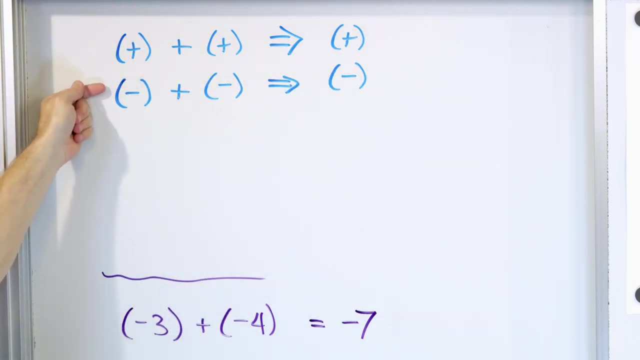 debt, two more in debt, three more in debt, four more in debt, I land on negative seven, which is what we said. So so far, positive plus positive always gives us positive, Negative plus negative always gives us negative, because when we add positive numbers, we're accumulating more money. 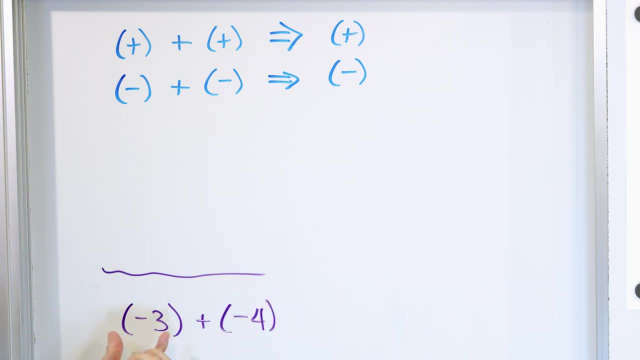 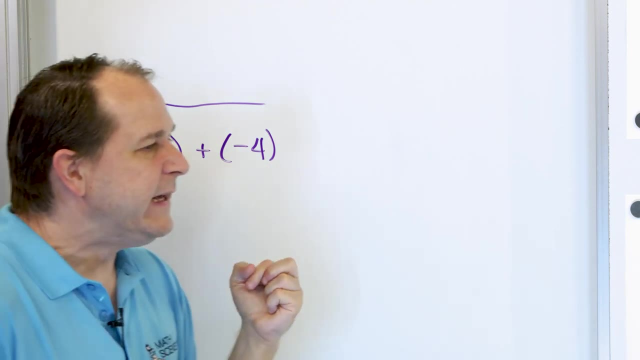 So it's, like I said, a negative plus a negative. So what does this mean? It means I start out by having a debt of three dollars. I owe somebody three dollars, but I add to that more debt, right, So I'm already in the hole because I've already owe somebody three dollars. 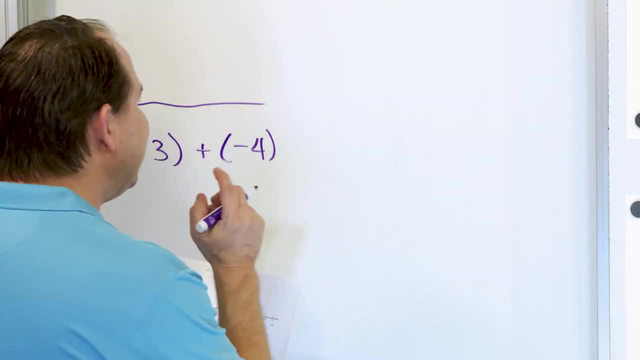 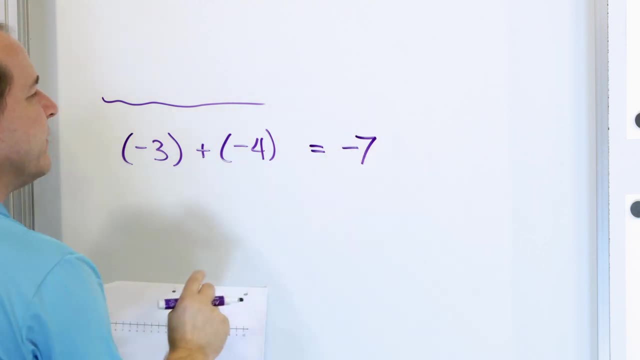 but then I have to go borrow more money for more dollars. So what do you think is going to be the answer? If I already owe three dollars and then I borrow four more dollars, I'm going to have a total debt of seven dollars. So negative plus negative always gives me a negative answer. 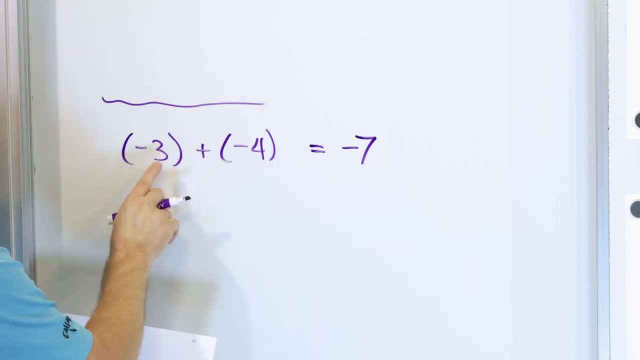 And notice what we did To get the number In our mind. we just took three plus four and made it seven. We still have to add the numbers, but because it's negative plus negative, which is debt plus debt, we kind of add. 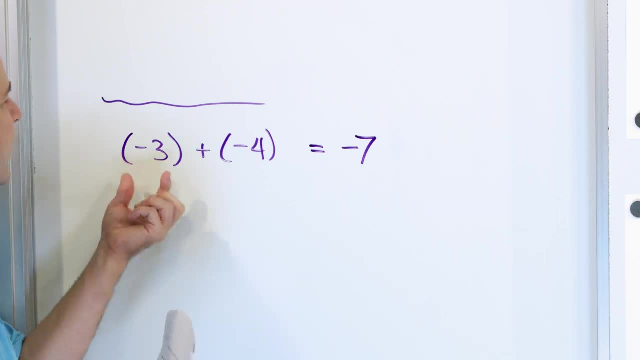 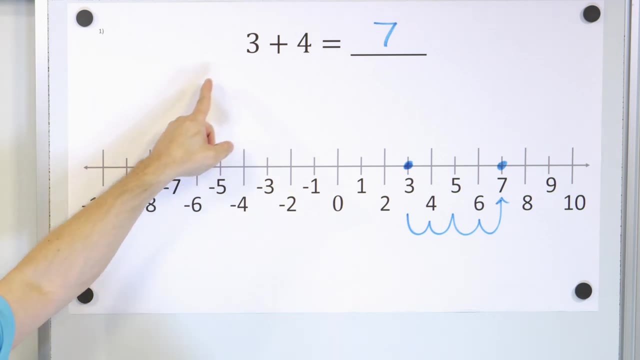 the numbers and then we just stick a negative sign on the front of it. So a negative plus another negative will always be a negative. If we were going to use the number line, then negative three plus negative four would mean that I would start at negative three, but I would be adding to it. 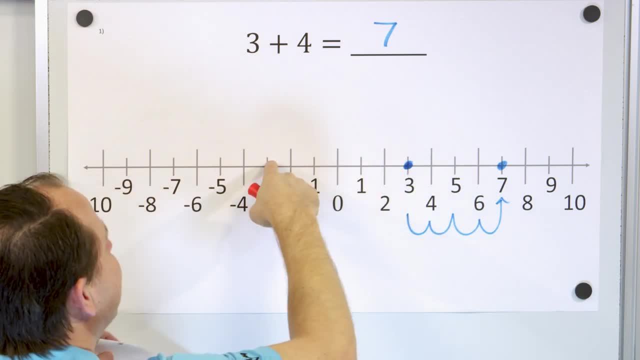 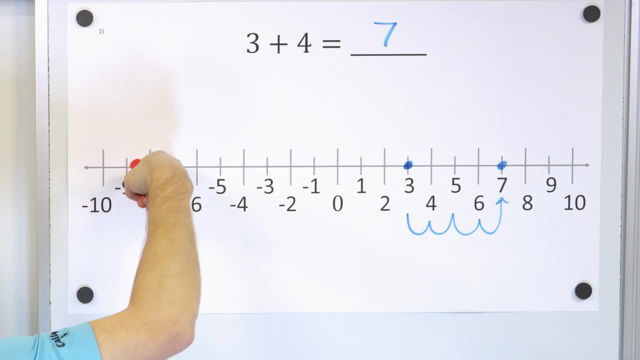 more debt. So I'm not going to go to the right because I'm not getting more money. I'm going to have to go to the left because I'm borrowing four dollars. One position, two position, three position, four positions: I land on negative seven. So, starting with negative three, going one more in. 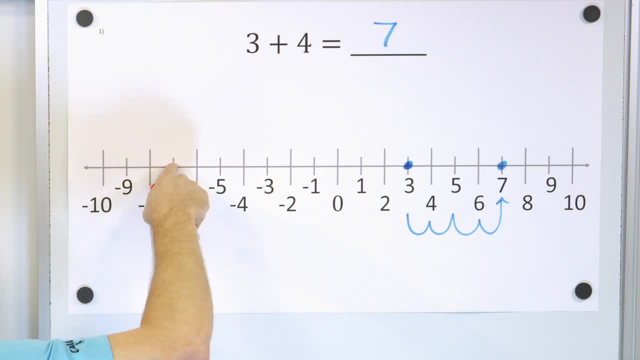 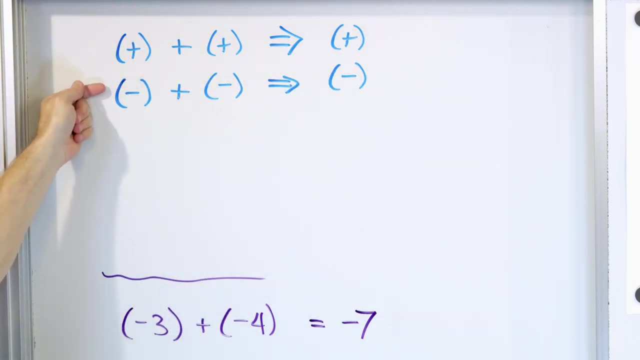 debt, two more in debt, three more in debt, four more in debt, I land on negative seven, which is what we said. So so far, positive plus positive always gives us positive, Negative plus negative always gives us negative, because when we add positive numbers, we're accumulating more money. 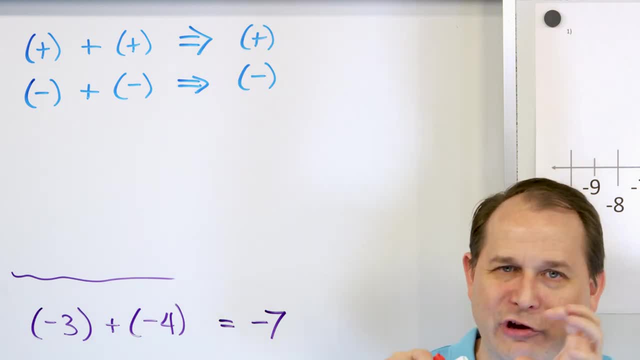 And if we're adding negative numbers, we start with debt and we're adding more debt. So those two are quite simple to understand when you think about it in terms of debt. Now, what happens if one of the numbers is positive and one of the numbers is negative and you try to add those? So there's really two cases. 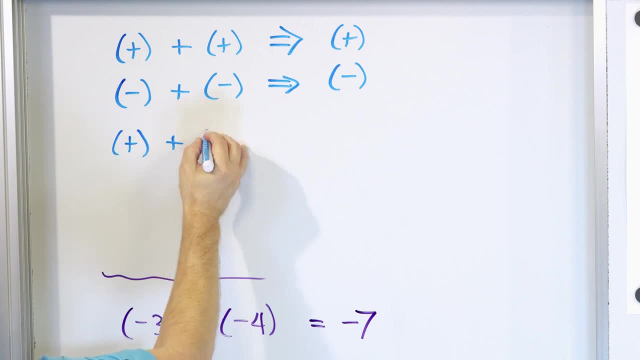 There is the case of: well, what if you start with a positive number and you add to it a negative number? Or what if you start with a negative number and you add to it a positive number? Well, actually, in this case what happens is you can either get a positive or a negative. 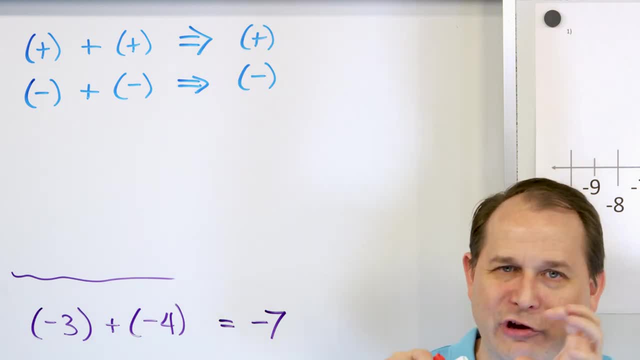 And if we're adding negative numbers, we start with debt and we're adding more debt. So those two are quite simple to understand when you think about it in terms of debt. Now, what happens if one of the numbers is positive and one of the numbers is negative and you try to add those? So there's really two cases. 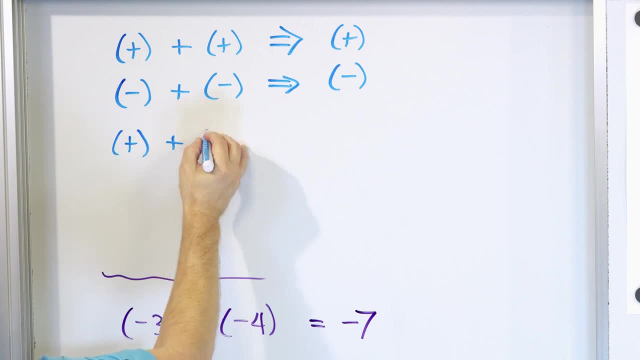 There is the case of: well, what if you start with a positive number and you add to it a negative number? Or what if you start with a negative number and you add to it a positive number? Well, actually, in this case what happens is you can either get a positive or a negative. 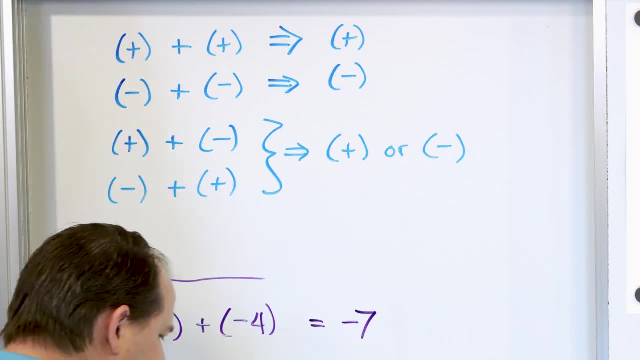 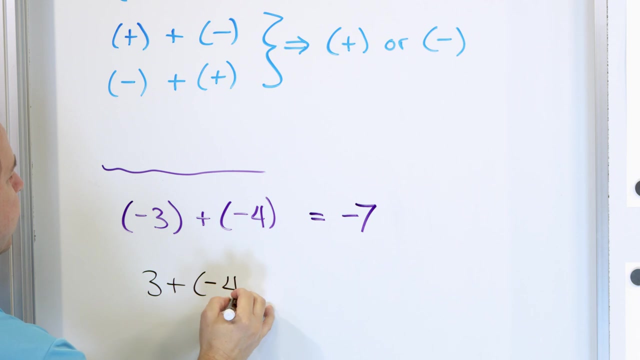 answer And it just depends on the problem that you have. It's going to be easier to explain in terms of of a concrete example. Let's say that I have, so we're doing positive plus negative. So instead of three, three plus four, let's make it three plus a negative four, right, So that's. 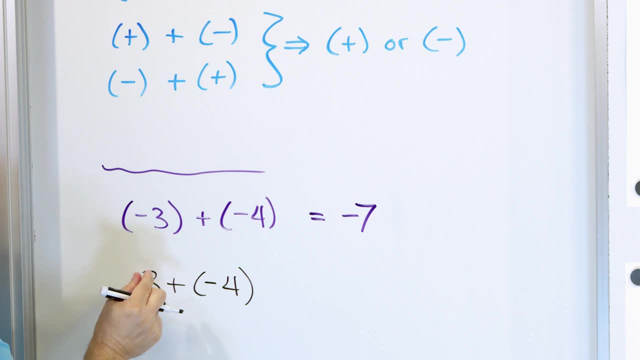 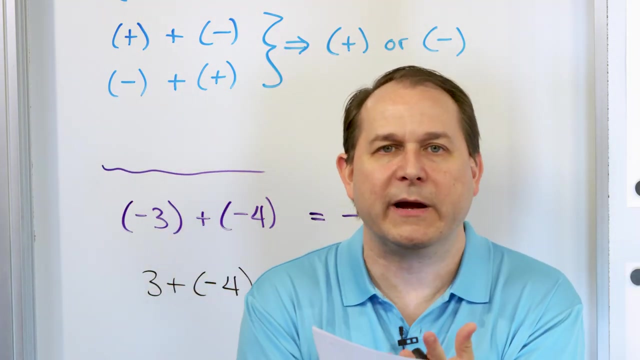 positive plus negative. So what does this mean? Actually, it means I start with $3 and instead of adding more money going to the right, I'm actually adding more debt. Think about it: If it $3, I had and I took on a debt of $3,. if I have $3 and I borrow $3, then I actually have no money. 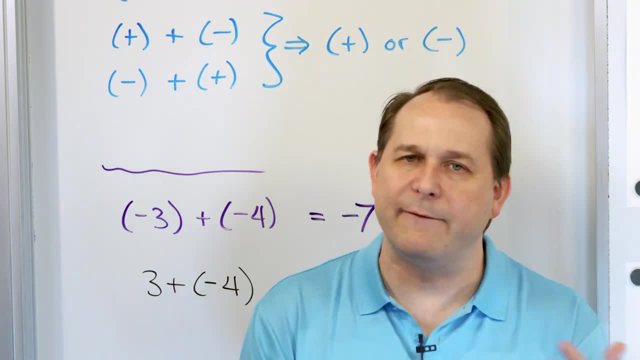 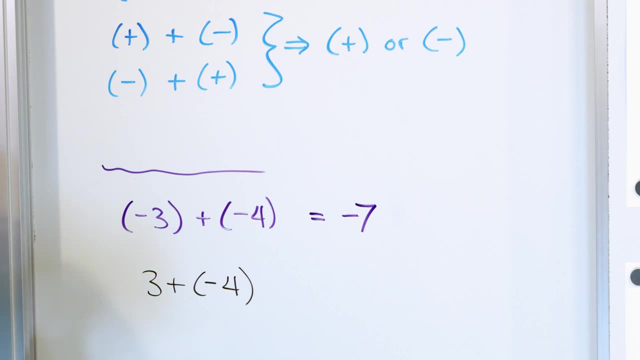 at all, because I use the money I have to pay my debt And then I'm left with nothing. But in this case I actually start with $3 and I borrow more money than I have. So you know from thinking about it logically that if I start with three and I borrow $4, I must still have a debt of 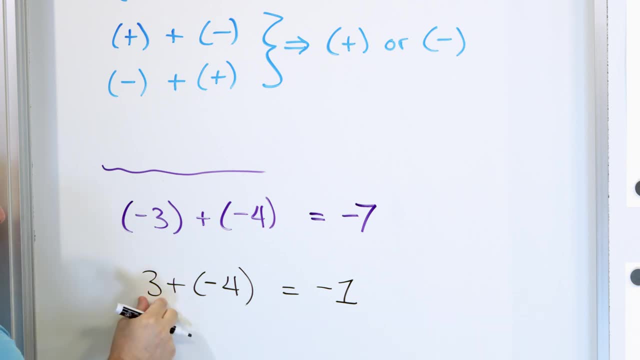 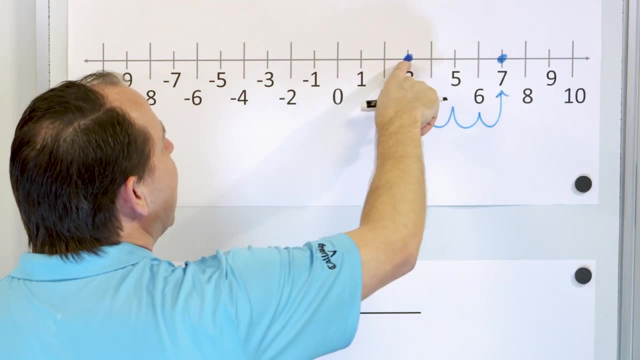 negative one at the end of it, because I only have three but I borrow four. So if I start on the number line with three and I add debt, it means I go four to the left. One more in debt, two more in debt, three more in debt- Now I have nothing. Four more in debt means: 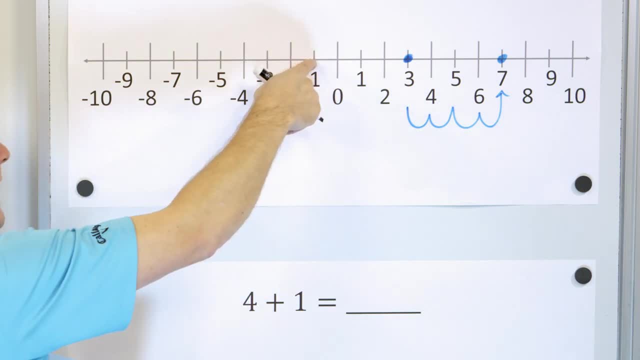 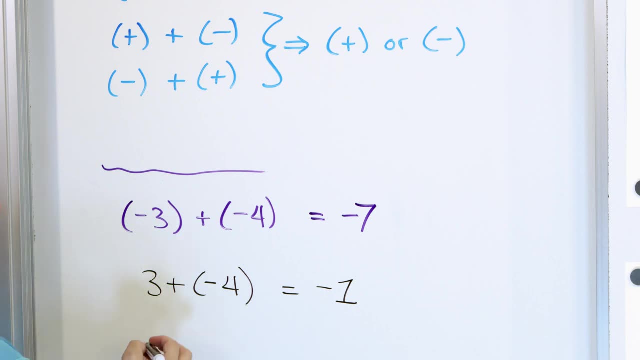 I have a debt at the end of it which is negative $1.. So the answer in this case was negative here. Now let's take a similar situation. Let's say we have negative four that we start with- I'm sorry, negative three that we start with. 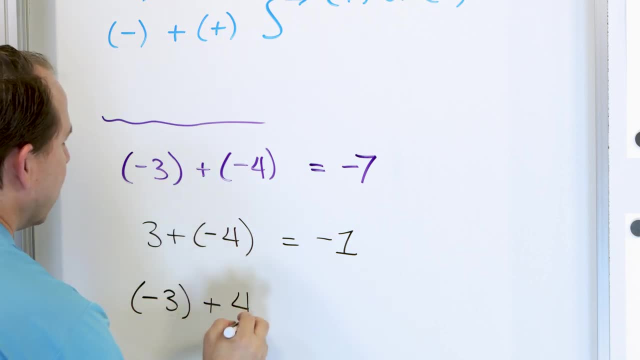 So we're doing negative plus positive. We're going to add to that a positive four. So we're going through all the cases. Here we had positive plus negative, Here we have negative plus positive. What's going to happen Now? think about it logically- If I start out being $3 in debt, 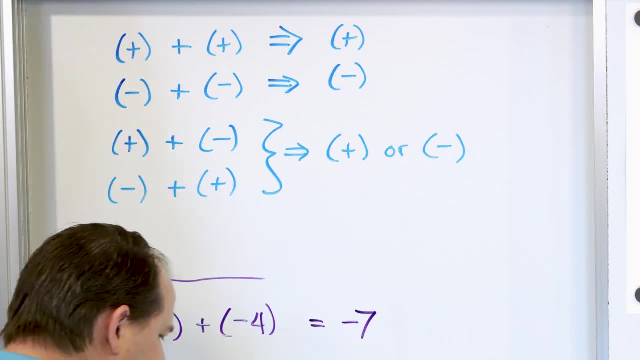 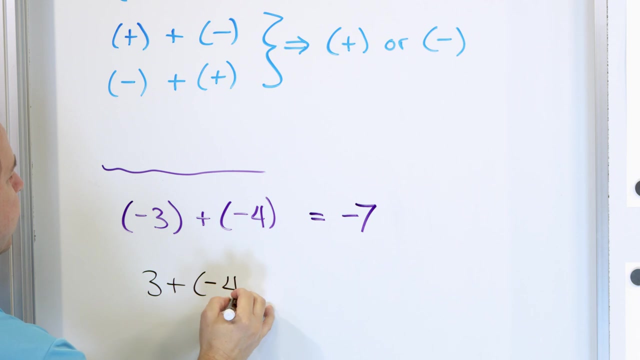 answer And it just depends on the problem that you have. It's going to be easier to explain in terms of of a concrete example. Let's say that I have, so we're doing positive plus negative. So instead of three, three plus four, let's make it three plus a negative four, right, So that's. 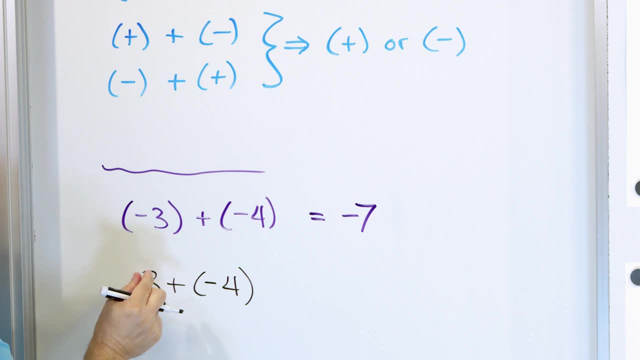 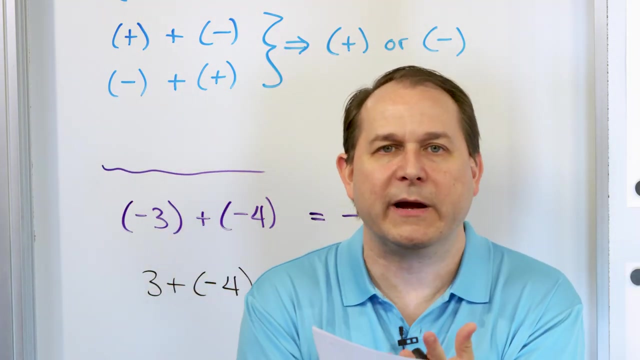 positive plus negative. So what does this mean? Actually, it means I start with $3 and instead of adding more money going to the right, I'm actually adding more debt. Think about it: If it $3, I had and I took on a debt of $3,. if I have $3 and I borrow $3, then I actually have no money. 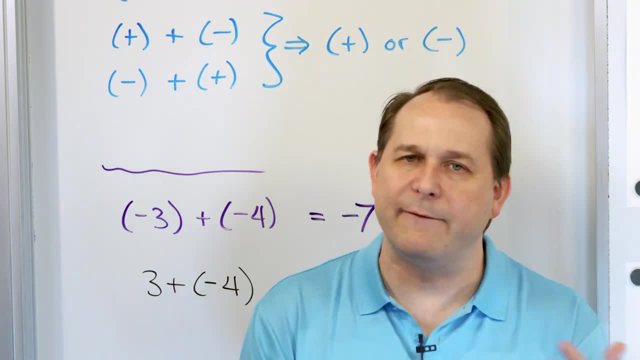 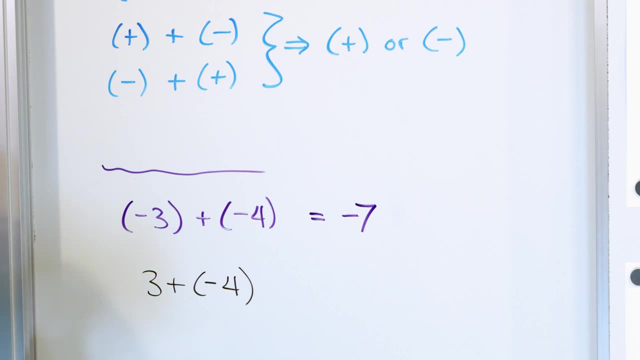 at all, because I use the money I have to pay my debt And then I'm left with nothing. But in this case I actually start with $3 and I borrow more money than I have. So you know from thinking about it logically that if I start with three and I borrow $4, I must still have a debt of 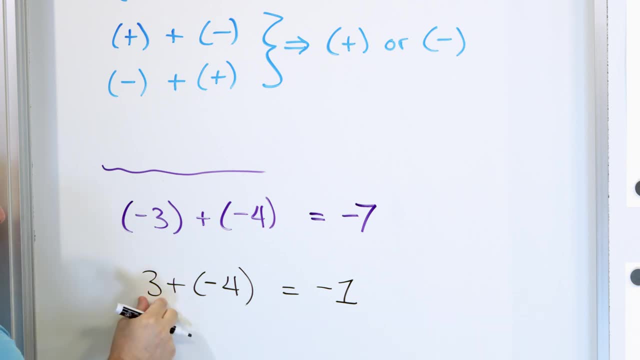 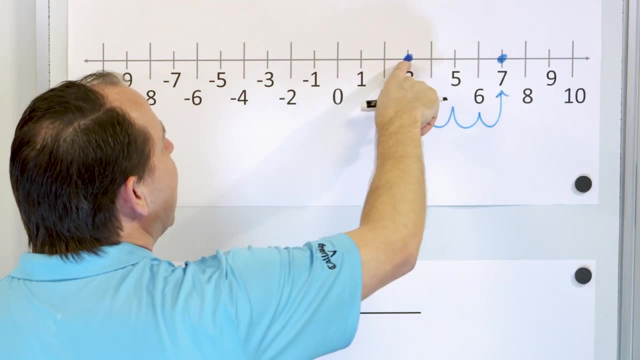 negative one at the end of it, because I only have three but I borrow four. So if I start on the number line with three and I add debt, it means I go four to the left. One more in debt, two more in debt, three more in debt- Now I have nothing. Four more in debt means: 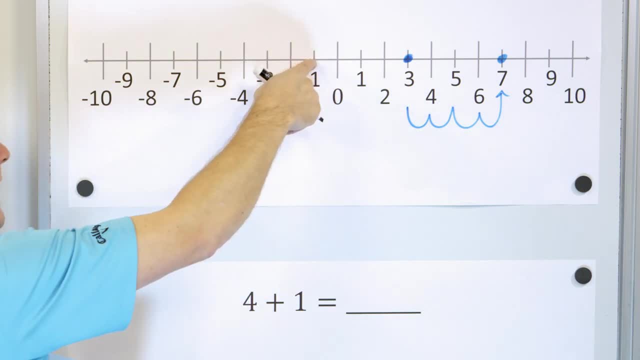 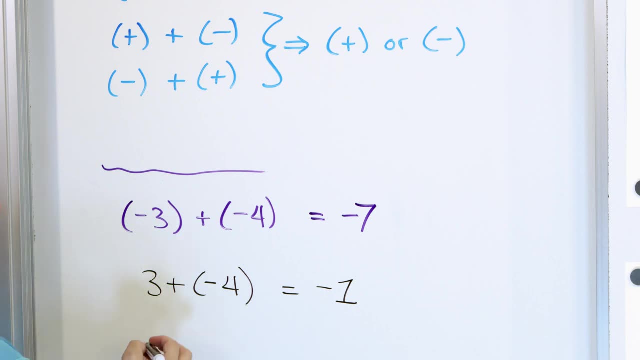 I have a debt at the end of it which is negative $1.. So the answer in this case was negative here. Now let's take a similar situation. Let's say we have negative four that we start with- I'm sorry, negative three that we start with. 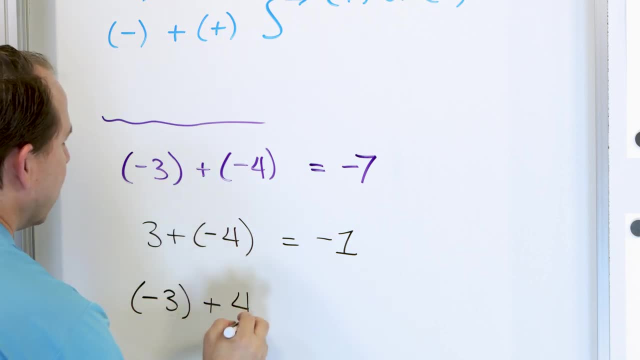 So we're doing negative plus positive. We're going to add to that a positive four. So we're going through all the cases. Here we had positive plus negative, Here we have negative plus positive. What's going to happen Now? think about it logically- If I start out being $3 in debt, 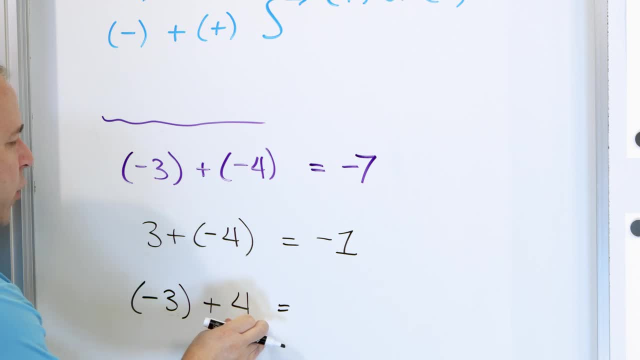 that's how much money I owe. And then someone gives me $4.. Well, I immediately pay my debt. I'm going to have $1 left. So the answer is a positive one, Because if I'm $3 in debt and I 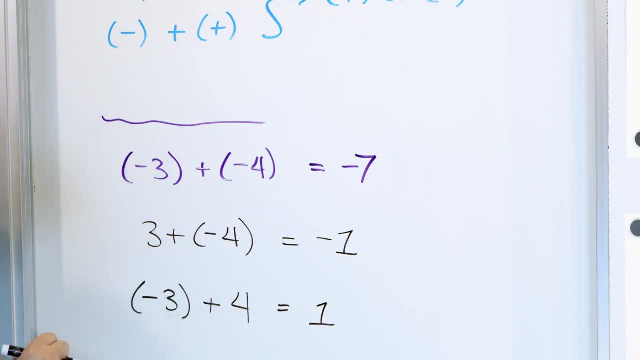 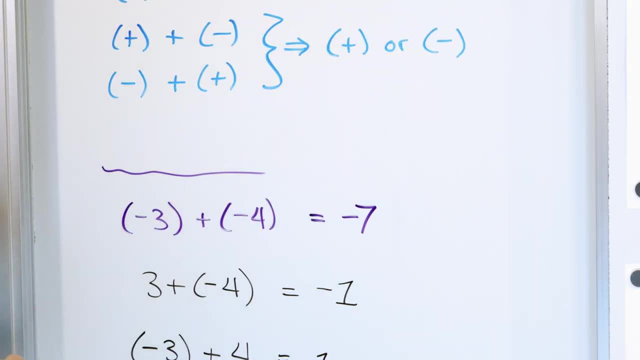 get more money. once I pay the debt off, I have $1 left over. So you see, when you have negative and positive plus negative, you can sometimes get negative answer and sometimes get a positive answer. If I start with $3 in debt and then someone gives me $4, I have to move to the right. 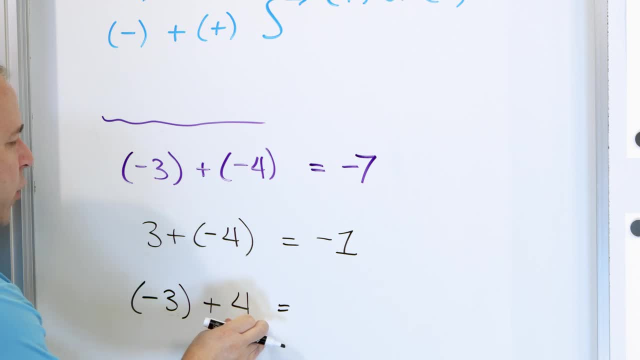 that's how much money I owe. And then someone gives me $4.. Well, I immediately pay my debt. I'm going to have $1 left. So the answer is a positive one, Because if I'm $3 in debt and I 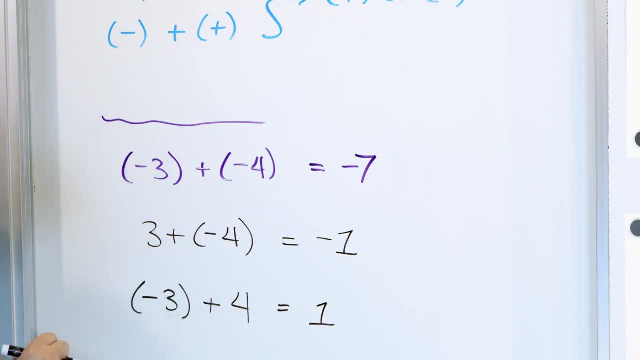 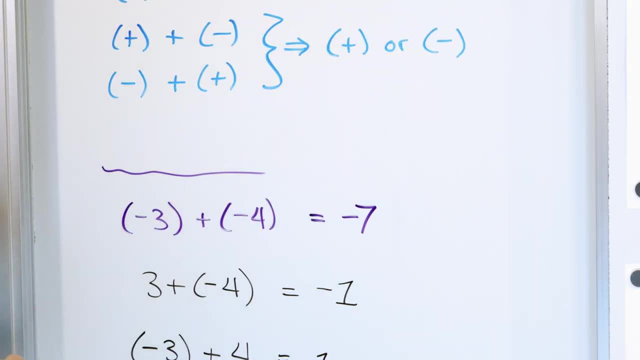 get more money. once I pay the debt off, I have $1 left over. So you see, when you have negative and positive plus negative, you can sometimes get negative answer and sometimes get a positive answer. If I start with $3 in debt and then someone gives me $4, I have to move to the right. 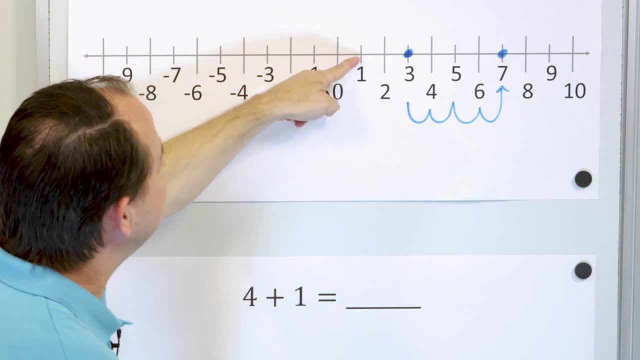 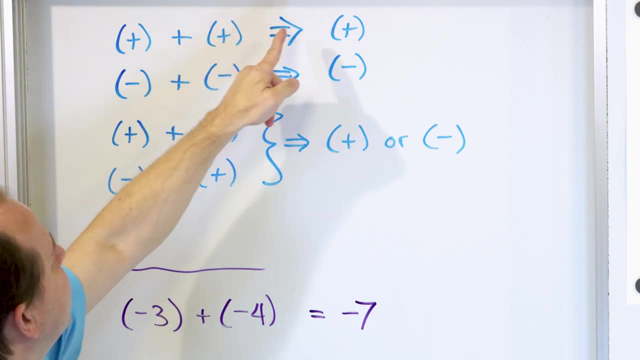 One, two, three, four And I land on $1.. That's how much money I have left after I do that. So the bottom line is: positive plus positive always gives me positive, Negative plus negative always gives us negative. But when you add two things where the signs are different, 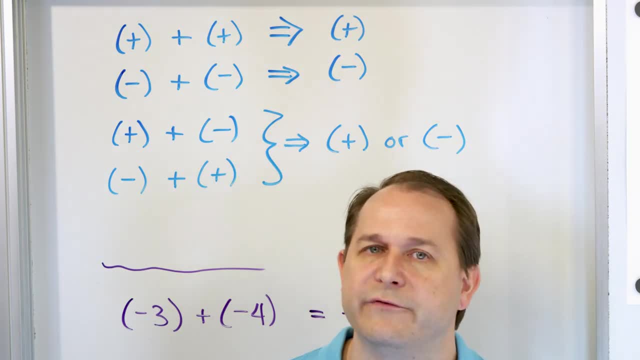 where it's either positive plus negative or negative plus positive, or negative plus negative, or negative plus positive. where the signs are different, then the answer you get can be either answer positive or negative. Now I want to tell you that we're going to be using these number. 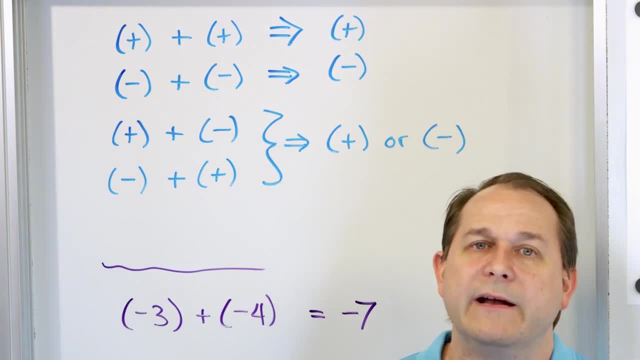 lines to solidify what we're doing. But let me show you the way I really think about this. And it's much easier than using number lines, because we have to take the training wheels off at some point with the number lines, right. So what happens if I'm adding positive to positive? 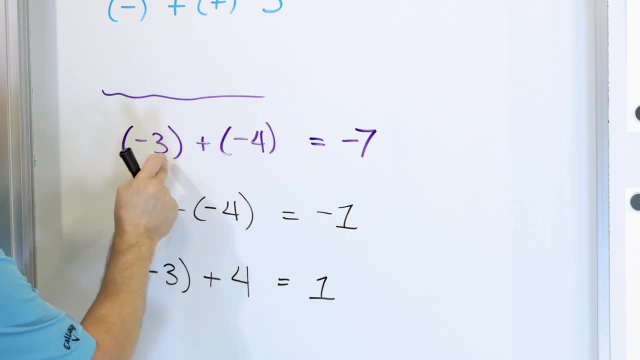 I add them like usual. If I add negative to negative, then of course I just add these numbers and stick a negative sign. But if I add two things that are different signs notice, positive to negative or negative to positive, they're different- Then what you do is you always subtract the numbers And then the sign. 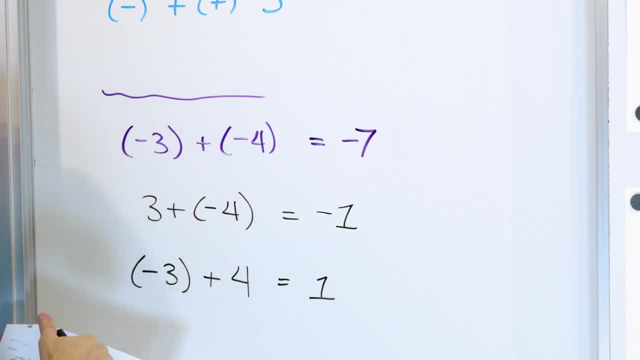 of the answer is just: whichever one of these is the bigger absolute value. So notice that you're adding different signs. So you just subtract the numbers: Four minus three is one And the sign of the answer is going to be negative because this is the one with the bigger absolute value. This 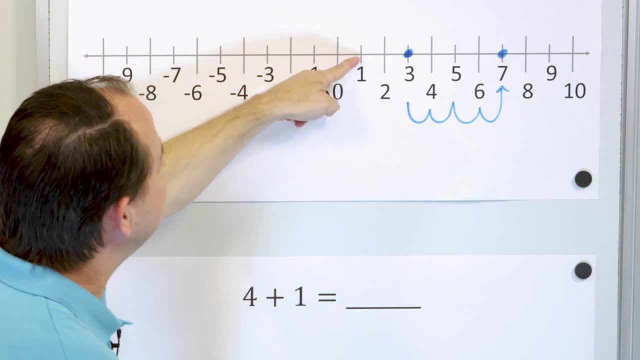 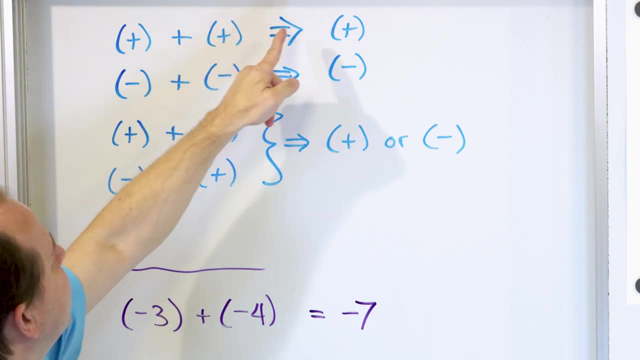 One, two, three, four And I land on $1.. That's how much money I have left after I do that. So the bottom line is: positive plus positive always gives me positive, Negative plus negative always gives us negative. But when you add two things where the signs are different, 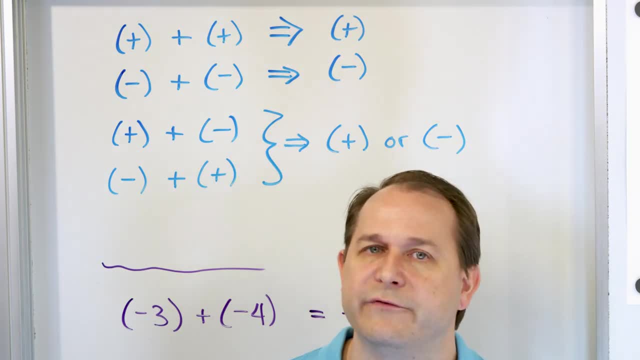 where it's either positive plus negative or negative plus positive, or negative plus negative, or negative plus positive. where the signs are different, then the answer you get can be either answer positive or negative. Now I want to tell you that we're going to be using these number. 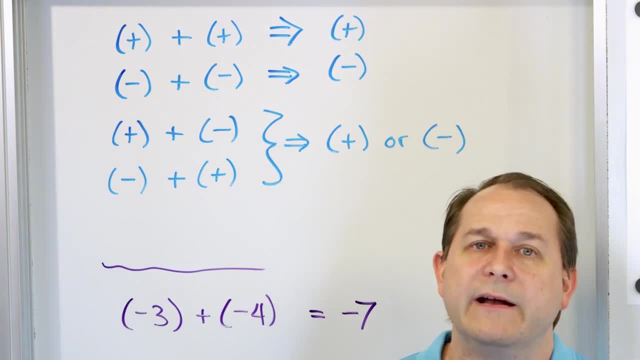 lines to solidify what we're doing. But let me show you the way I really think about this. And it's much easier than using number lines, because we have to take the training wheels off at some point with the number lines, right. So what happens if I'm adding positive to positive? 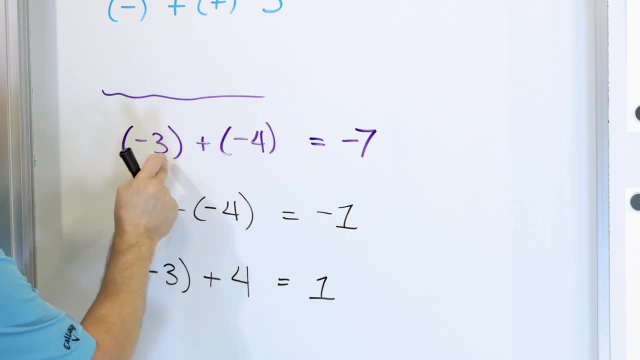 I add them like usual. If I add negative to negative, then of course I just add these numbers and stick a negative sign. But if I add two things that are different signs notice, positive to negative or negative to positive, they're different- Then what you do is you always subtract the numbers And then the sign. 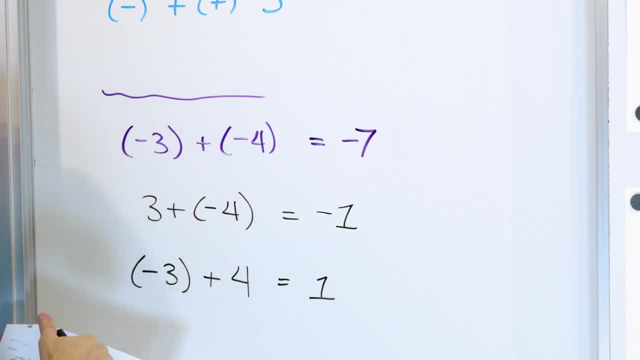 of the answer is just: whichever one of these is the bigger absolute value. So notice that you're adding different signs. So you just subtract the numbers: Four minus three is one And the sign of the answer is going to be negative because this is the one with the bigger absolute value. This 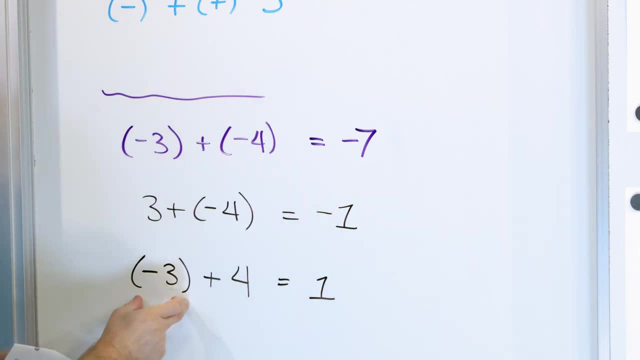 one has more worth, And so the sign is negative. We're adding different signs, And anytime they're different. you just subtract them. Four minus three is one, And the sign of the answer is going to be positive, because this is the one that has the 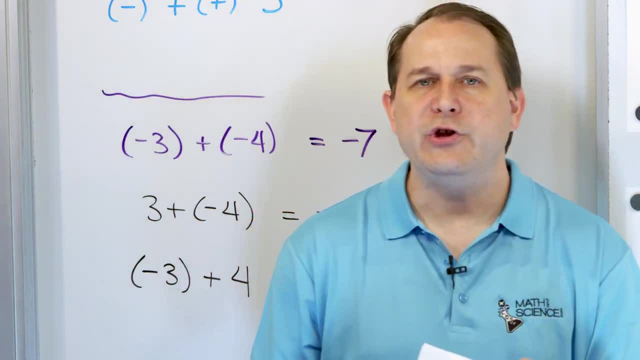 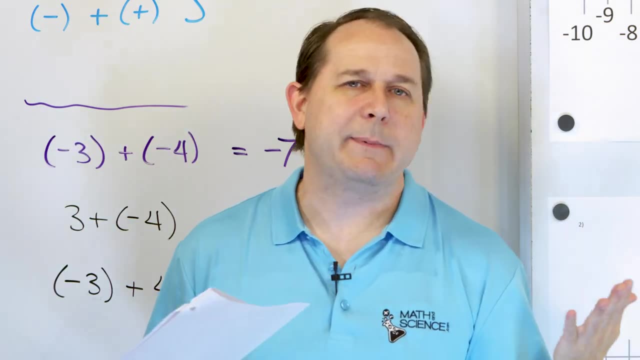 bigger absolute value. Why does it work this way? Because when you have a positive number and a negative number, they're like matter and antimatter: They try to kill each other. okay, So think about it this way: If you had $4, that's positive four, And I add to that a debt. 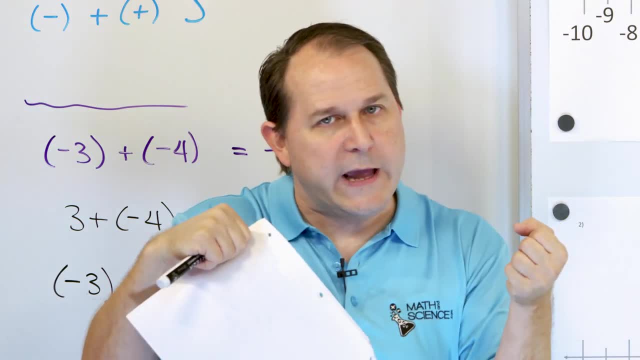 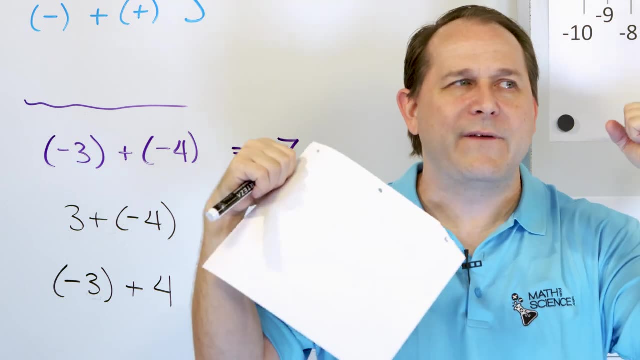 of negative four. It's like one of those numbers is pulling one way and the other one is pulling the other way, Because one's positive, that's money you have, And the other one's negative, that's money you owe. So if I have positive and negative four, they just cancel out and I have zero Once I pay the debt. 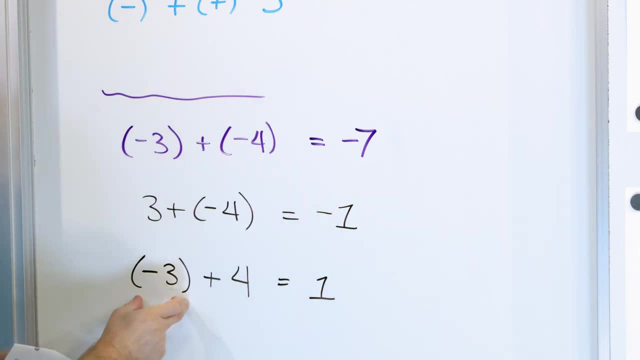 one has more worth, And so the sign is negative. We're adding different signs, And anytime they're different. you just subtract them. Four minus three is one, And the sign of the answer is going to be positive, because this is the one that has the 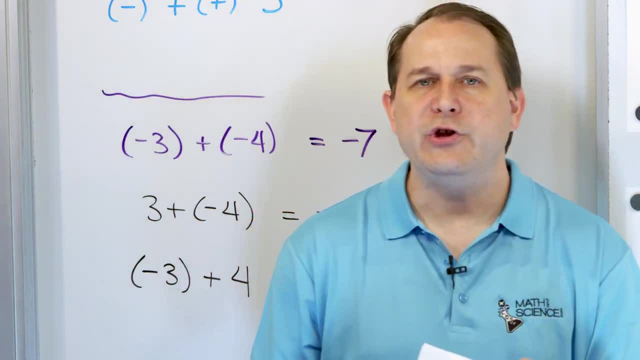 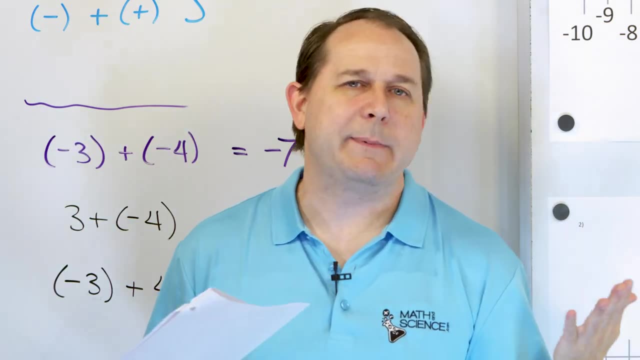 bigger absolute value. Why does it work this way? Because when you have a positive number and a negative number, they're like matter and antimatter: They try to kill each other. okay, So think about it this way: If you had $4, that's positive four, And I add to that a debt. 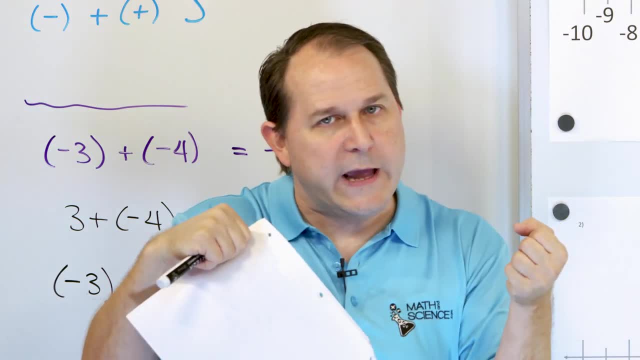 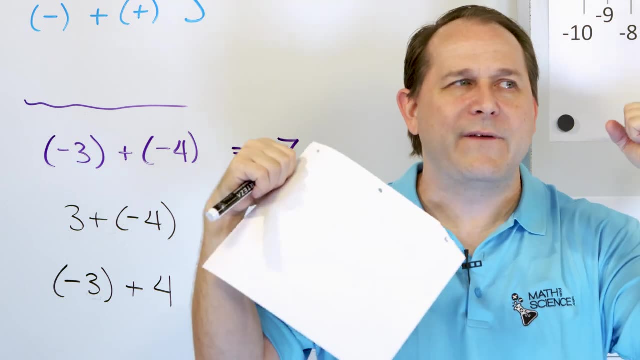 of negative four. It's like one of those numbers is pulling one way and the other one is pulling the other way, Because one's positive, that's money you have, And the other one's negative, that's money you owe. So if I have positive and negative four, they just cancel out and I have zero Once I pay the debt. 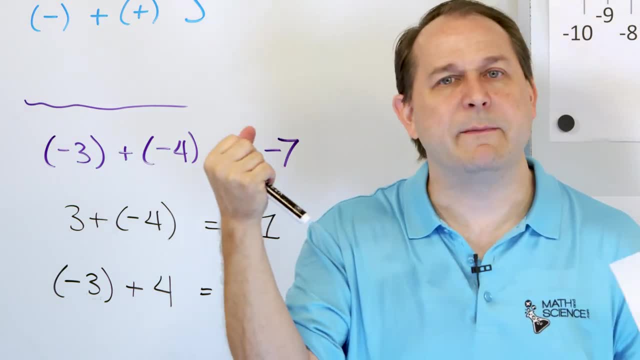 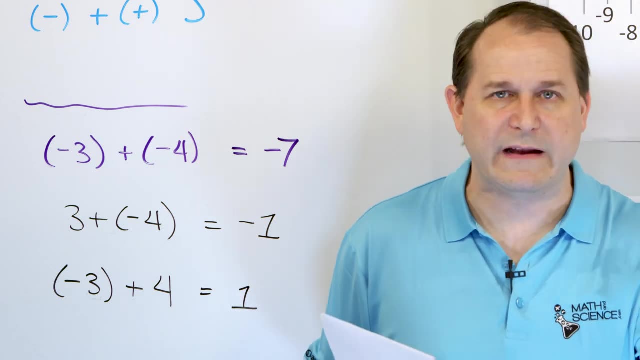 I have nothing left. But if the positive number is the bigger number, then the sign of the answer is going to be positive, because that's more of what you have. If the negative number is the one that's bigger, then the sign of the answer will be debt negative, because that's the one that 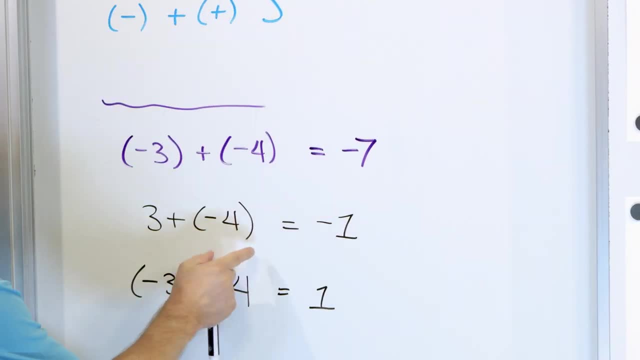 you have more, of more debt. So in this problem we had more debt, So the answer had to be negative. once they collided with each other Here, the bigger number was positive. I had more money, so the answer had to be positive, But in both cases I just subtracted. 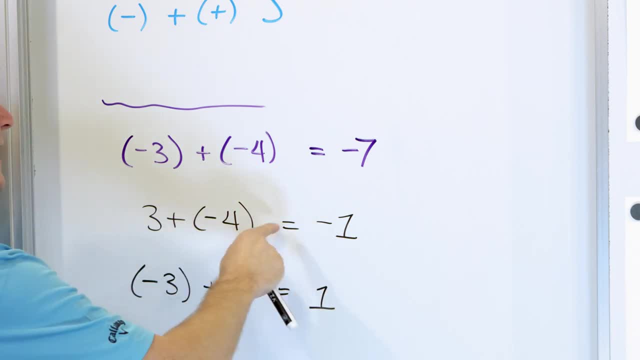 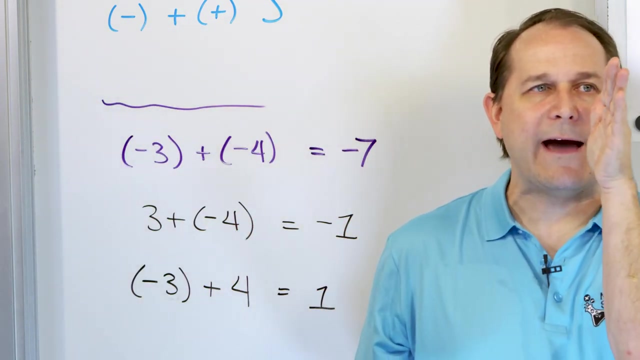 four minus three And four minus three, I get one. But the sign here has to be negative because I had more debt in the problem And the sign of this one had to be positive because I had more positive money in the problem. So bottom line, as we solve these when we have opposite signs- negative plus- 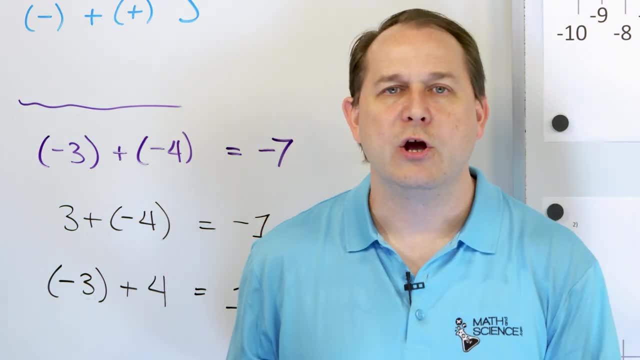 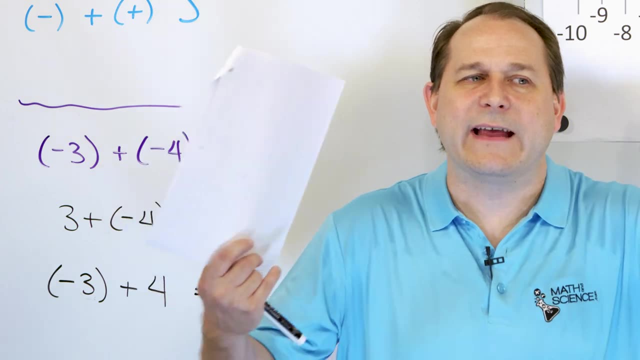 positive or positive plus negative. we have a negative sign, And the sign of this one has to be negative. We're going to do the same thing every time. We're going to subtract the numbers every time, But the sign of the answer will just be: whatever is the bigger absolute value. It's like 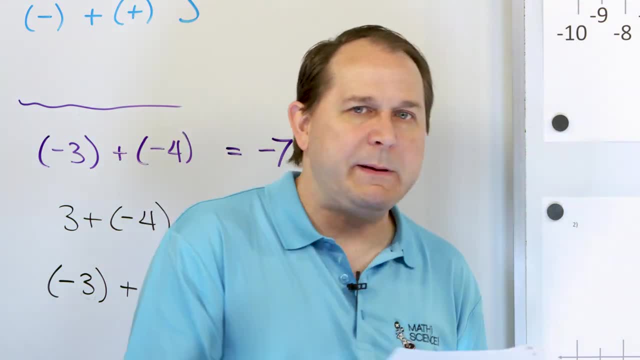 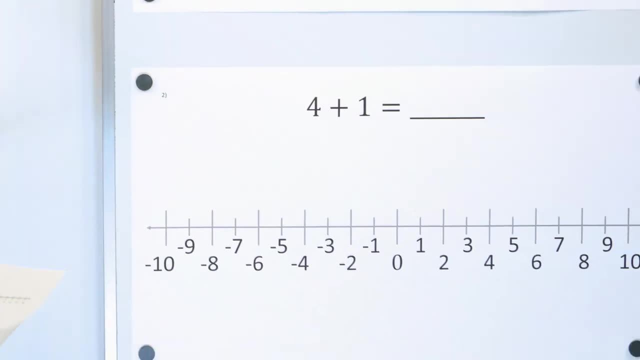 which one is the winner in the tug of war. Is the positive one going to be pulling more or the negative one being pulling more? That's the one that will give you the correct sign of the answer. All right, So let's move along to problem number two. So here we have positive plus positive. 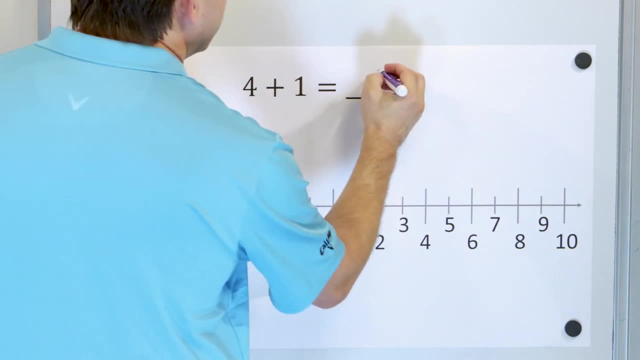 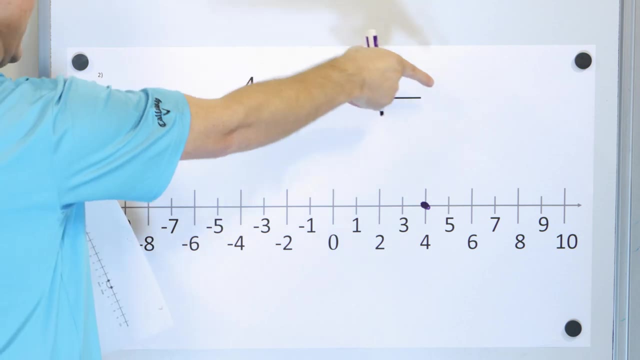 That's what we all know from third grade. That's going to be five. Four plus one is five. Why? Because if I start with four dollars and I go up to the right one unit, I'm going to land on five dollars. So I move to the right whenever I add positive numbers like that. So four plus one is 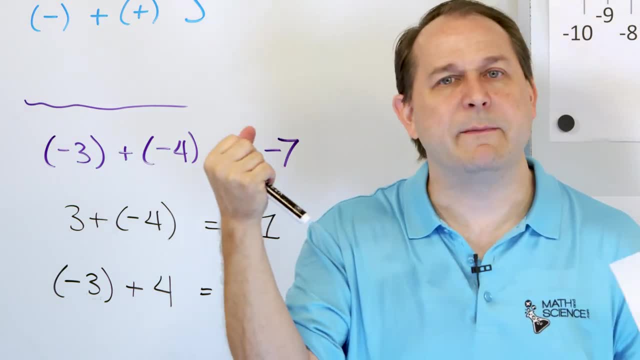 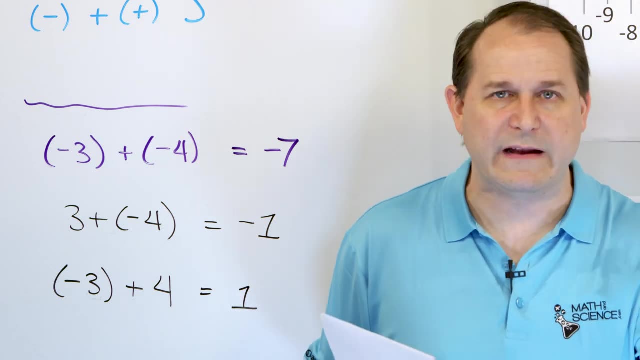 I have nothing left. But if the positive number is the bigger number, then the sign of the answer is going to be positive, because that's more of what you have. If the negative number is the one that's bigger, then the sign of the answer will be debt negative, because that's the one that 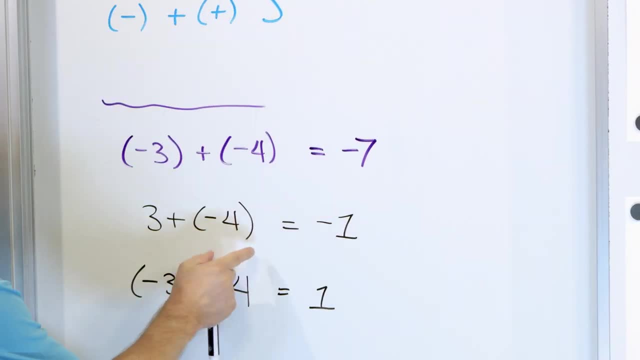 you have more, of more debt. So in this problem we had more debt, So the answer had to be negative. once they collided with each other Here, the bigger number was positive. I had more money, so the answer had to be positive, But in both cases I just subtracted. 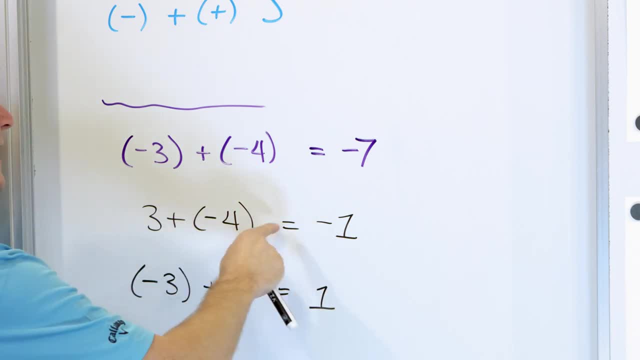 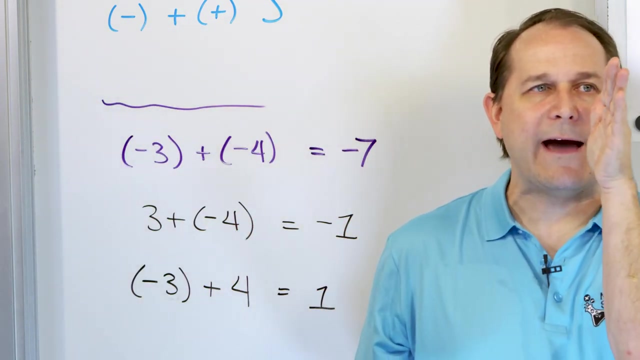 four minus three And four minus three, I get one. But the sign here has to be negative because I had more debt in the problem And the sign of this one had to be positive because I had more positive money in the problem. So bottom line, as we solve these when we have opposite signs- negative plus- 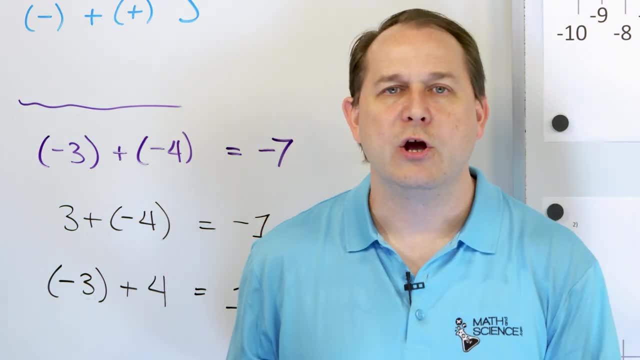 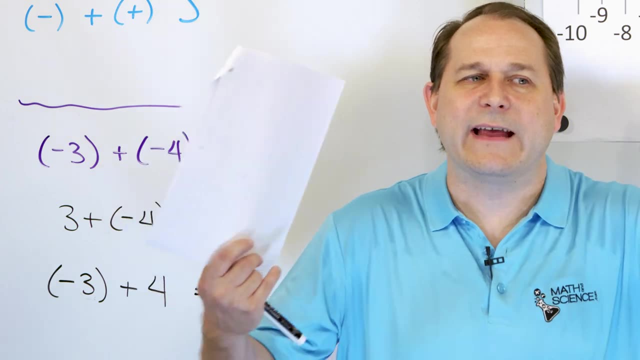 positive or positive plus negative. we're going to have negative plus positive. So what? we're going to negative? we're going to do the same thing every time. We're going to subtract the numbers every time, but the sign of the answer will just be: whatever is the bigger absolute value. It's like 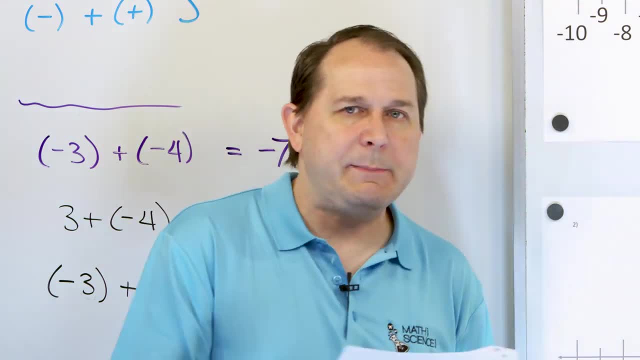 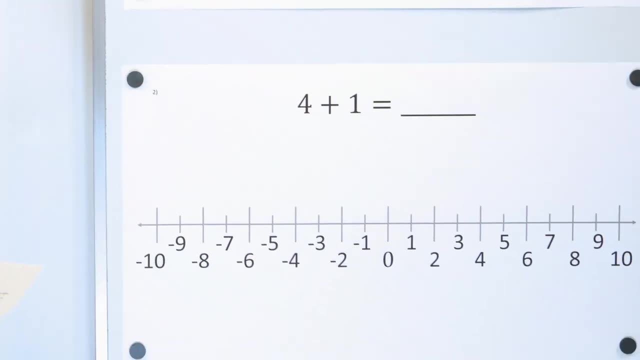 which one is the winner in the tug of war. Is the positive one going to be pulling more or the negative one being pulling more? That's the one that will give you the correct sign of the answer. All right, So let's move along to problem number two. So here we have positive plus positive. 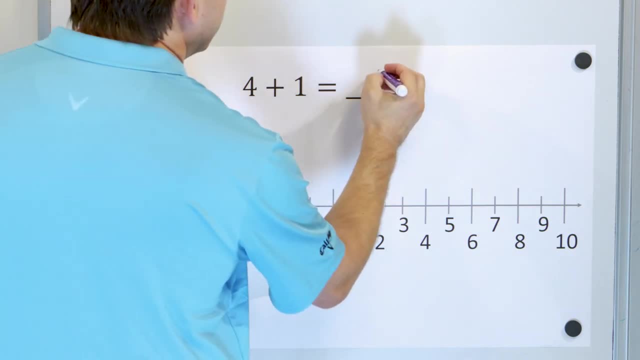 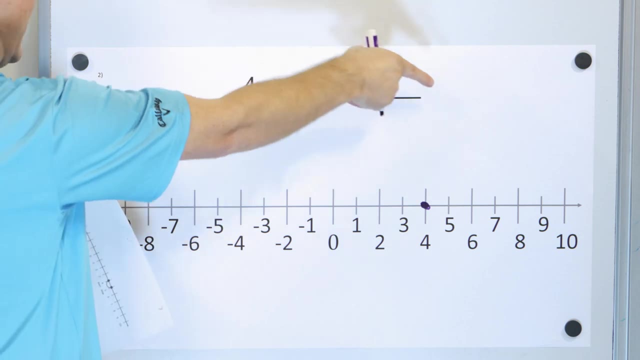 That's what we all know from third grade. That's going to be five. Four plus one is five. Why? Because if I start with four dollars and I go up to the right one unit, I'm going to land on five dollars. So I move to the right whenever I add positive numbers like that. So four plus one is 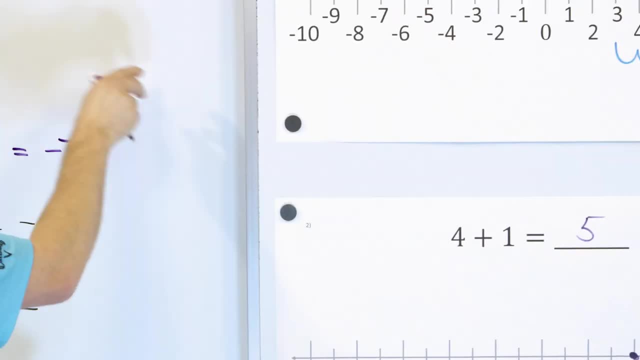 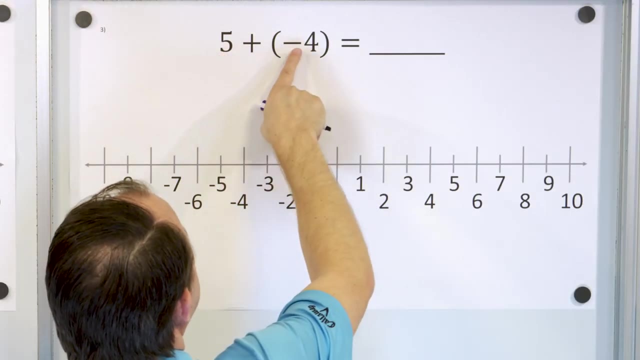 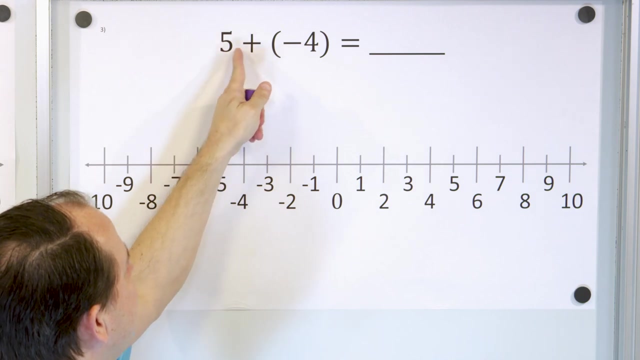 five, All right. So that's this case. right here, Positive plus positive always gives you positive. Now here is a case where I have positive plus negative. Remember anytime you have opposite signs and you're adding them like this, And so this is positive plus negative. 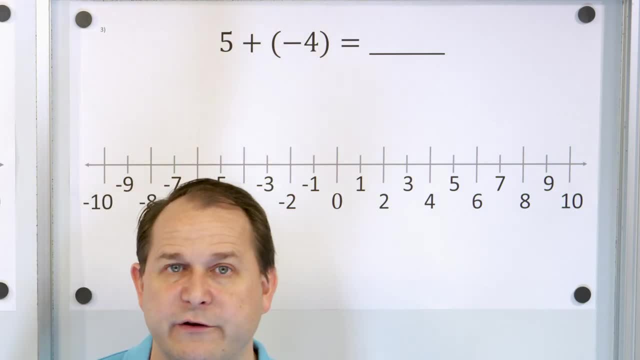 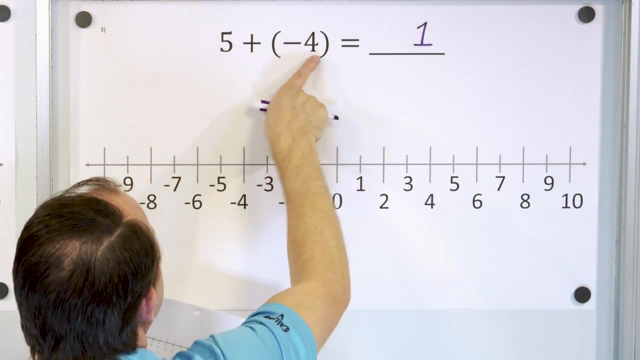 And this is negative and you're adding them. Then the fast way to do it is you just always subtract the numbers. Five minus four is just going to give you one, And the sign of it is always going to be which one of these is bigger. I have more money than debt. This one is the bigger. 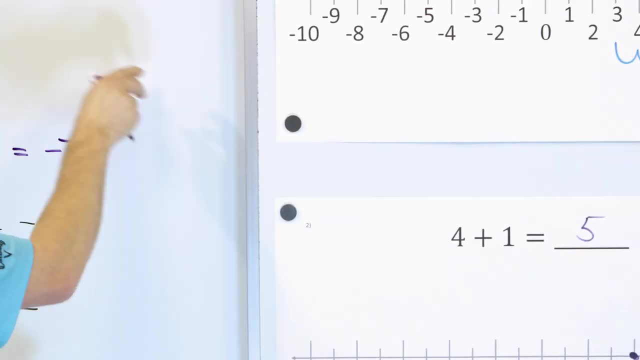 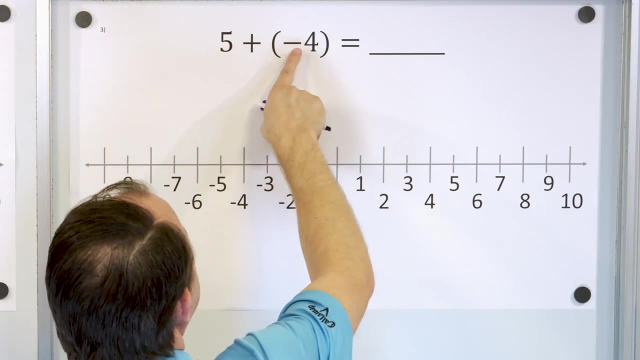 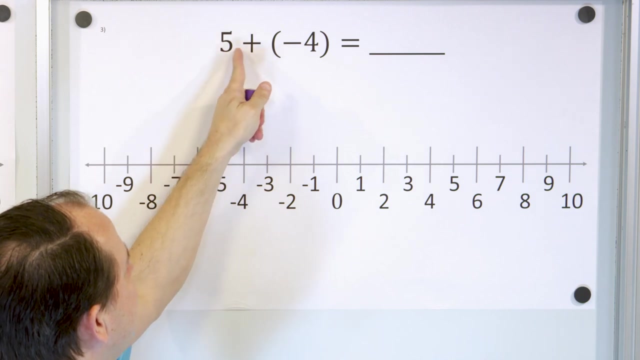 five, All right. So that's this case. right here, Positive plus positive always gives you positive. Now here is a case where I have positive plus negative. Remember any time you have opposite signs and you're adding them like this, And so this is positive plus negative, And I'm going to. 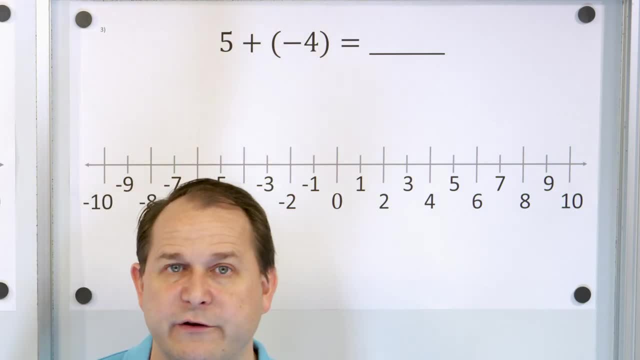 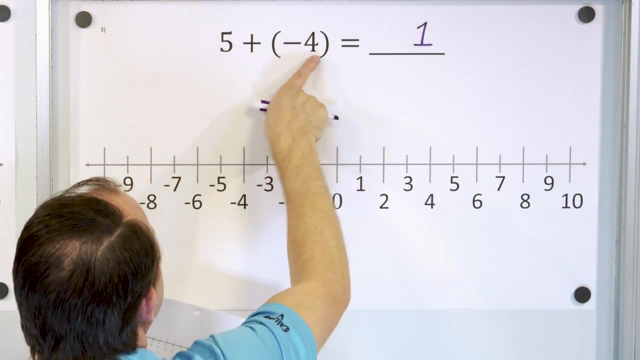 and this is negative and you're adding them, Then the fast way to do it is you just always subtract the numbers. Five minus four is just going to give you one, And the sign of it is always going to be which one of these is bigger. I have more money than debt. This one is the bigger. 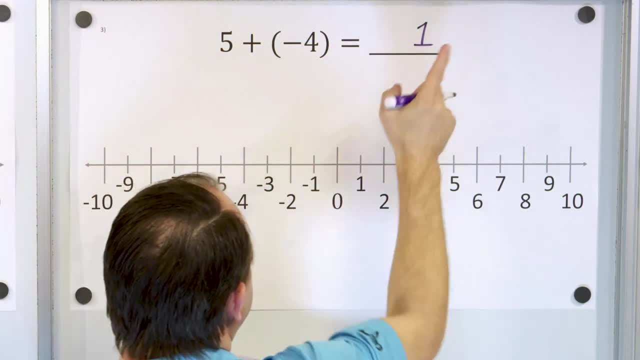 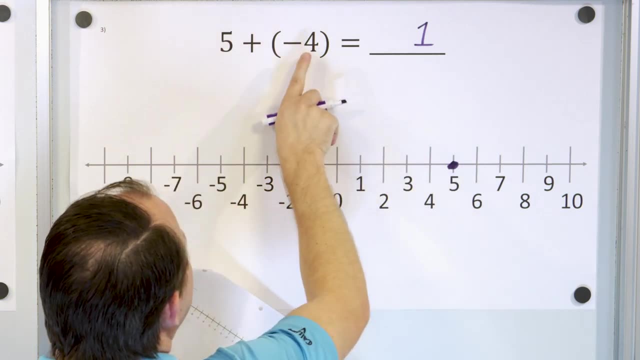 absolute value. So the answer is positive, Right, And so the answer is positive one. That's the answer, And you can think about it by saying that you start with five dollars and by adding more debt, you can't go to the right. The debt makes you go to the left. four units Two. 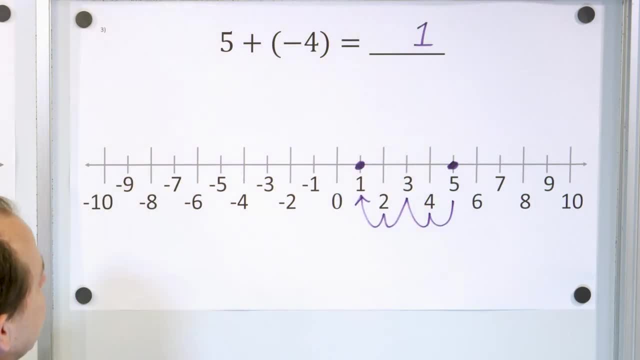 three, four And you land on a positive one. That's the answer, Right? So just subtract the numbers. Five minus four is one, And the sign goes with the bigger of the absolute value. In this case it's positive. Now you can also think about from the last lesson, if it helps you. 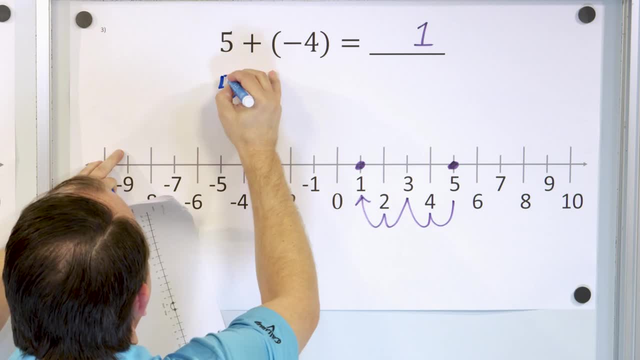 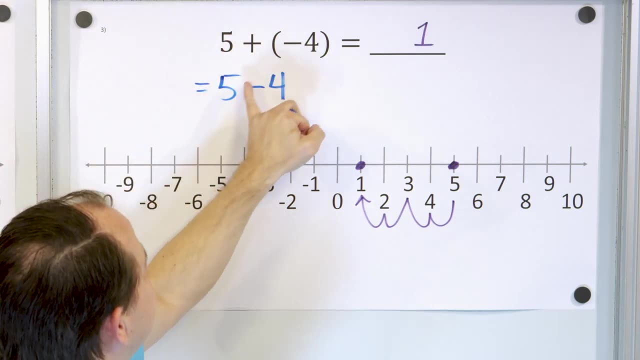 when we have a plus minus, like that, you can write it a subtraction: Five minus four, Right, So these are the same thing. You could say it's five minus four, which is one. So if it's easier for you to write this as subtraction and say five minus four is one, that's fine. But I want you to start. 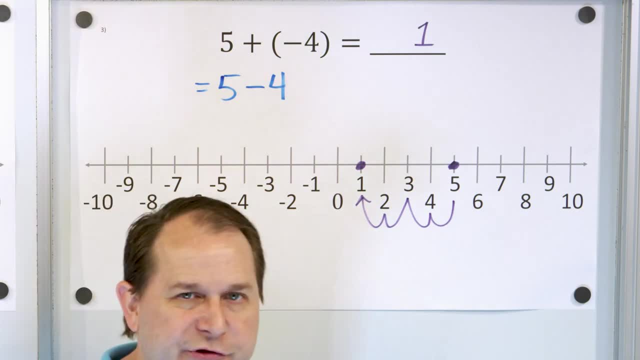 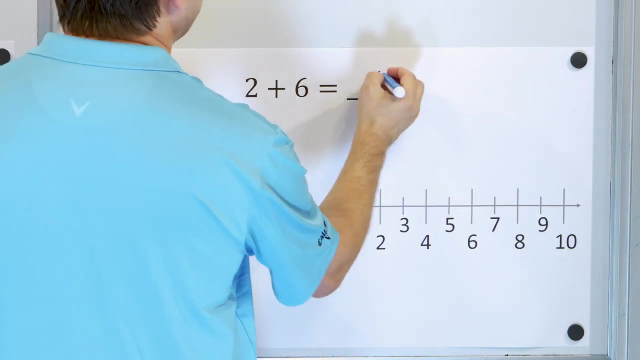 about adding negative numbers and which one is larger, because which one is larger is going to tell you what the sign of the answer is when the signs are opposites. All right, Let's take a look at problem number four here. Two plus six Positive plus positive always gives us positive. 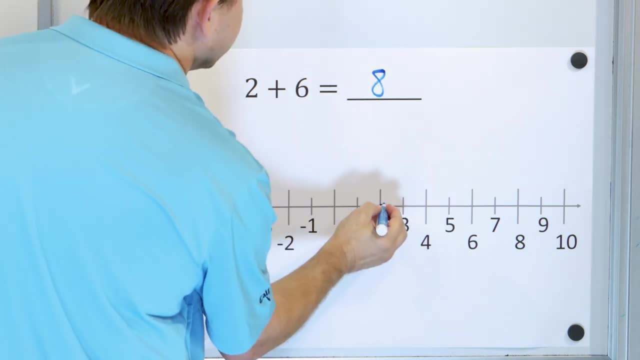 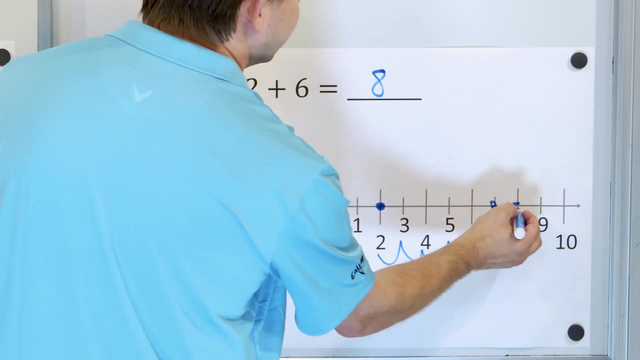 And we add them, of course, and we get an eight. If we start with two and we add six, we go to the right: One, two, three, four, five, six, And so we land on eight. Whoops, not seven, eight, Sorry. 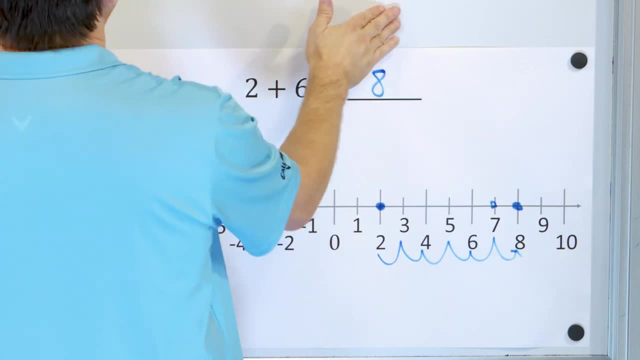 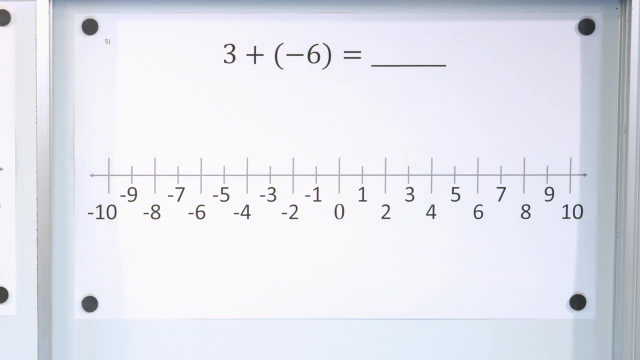 should be eight, And so two plus six is eight. Positive plus positive is positive, as we have said before. Now here we have a situation where we have a positive plus a negative. They're opposite signs. So the fast way to do it is just to say: OK, I'm adding something. 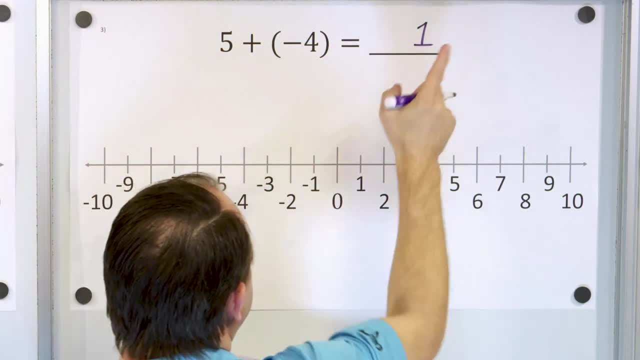 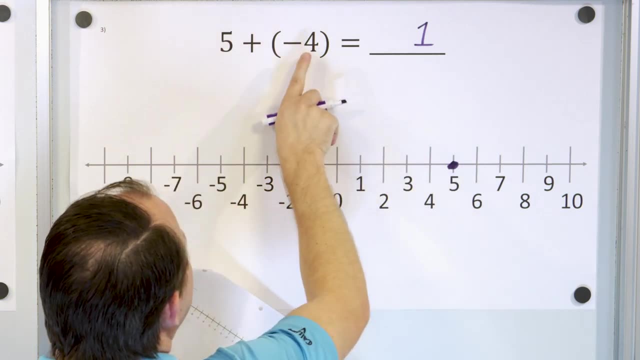 absolute value. So the answer is positive, Right, And so the answer is positive one. That's the answer, And you can think about it by saying that you start with five dollars and by adding more debt, you can't go to the right. The debt makes you go to the left. four units Two. 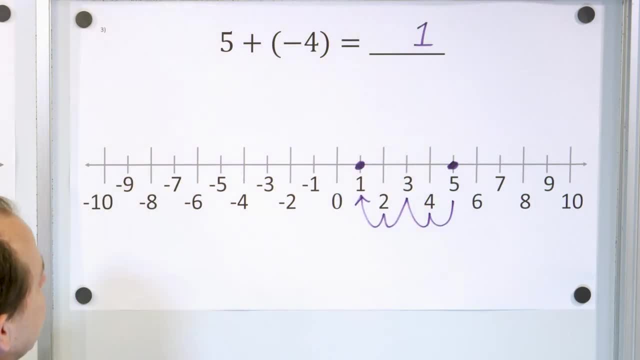 three, four And you land on a positive one. That's the answer, Right? So just subtract the numbers. Five minus four is one, And the sign goes with the bigger of the absolute value. In this case it's positive. Now you can also think about from the last lesson, if it helps you. 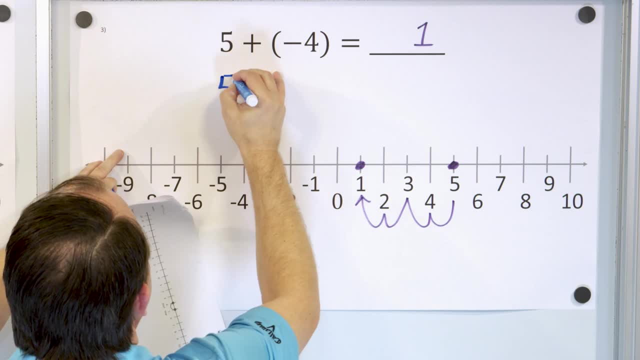 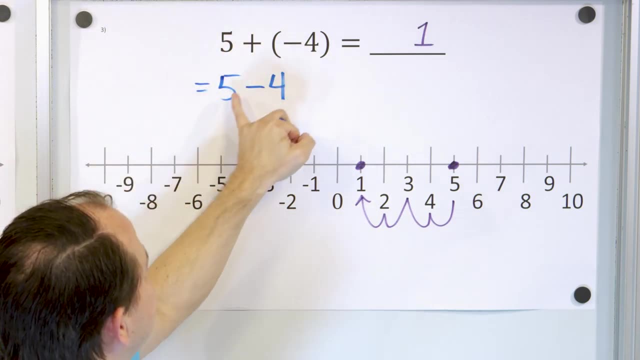 when we have a plus minus, like that, you can write it a subtraction: Five minus four, Right, So these are the same thing. You could say it's five minus four, which is one. So if it's easier for you to write this as subtraction and say five minus four is one, that's fine. But I want you to start. 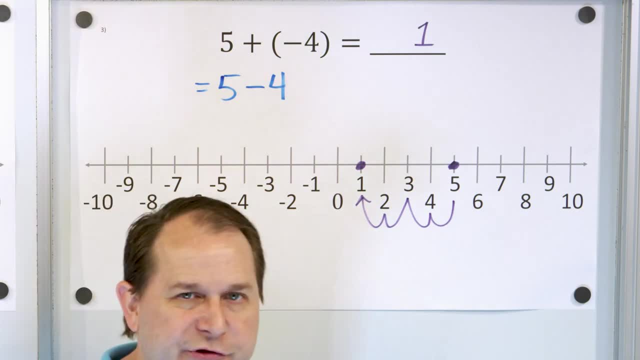 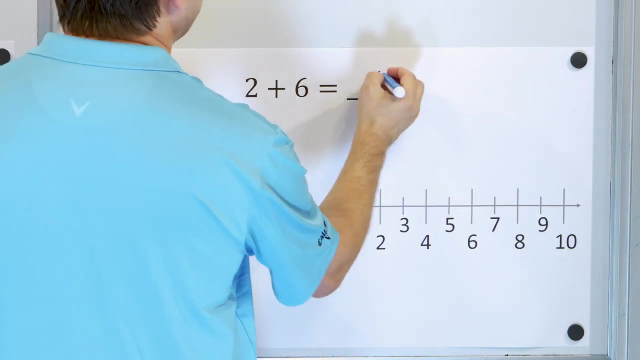 about adding negative numbers and which one is larger, because which one is larger is going to tell you what the sign of the answer is when the signs are opposites. All right, Let's take a look at problem number four here. Two plus six Positive plus positive always gives us positive. 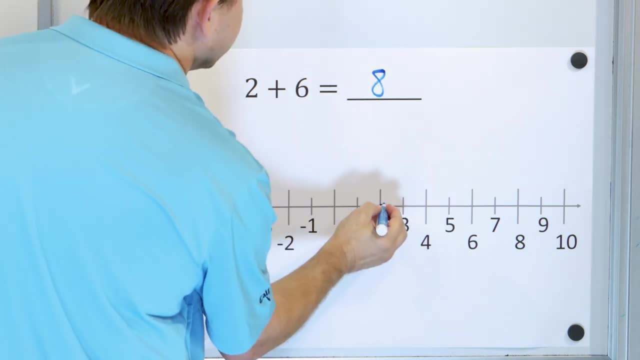 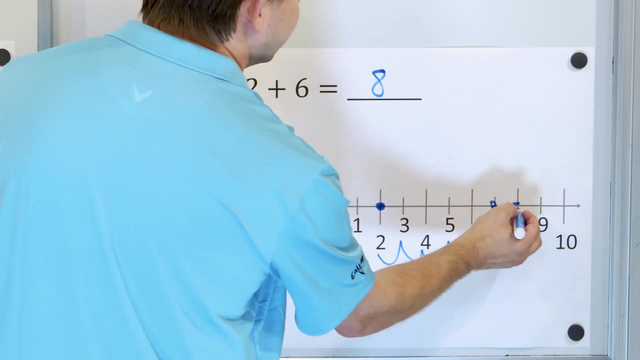 And we add them, of course, and we get an eight. If we start with two and we add six, we go to the right: One, two, three, four, five, six, And so we land on eight. Whoops, not seven, eight, Sorry. 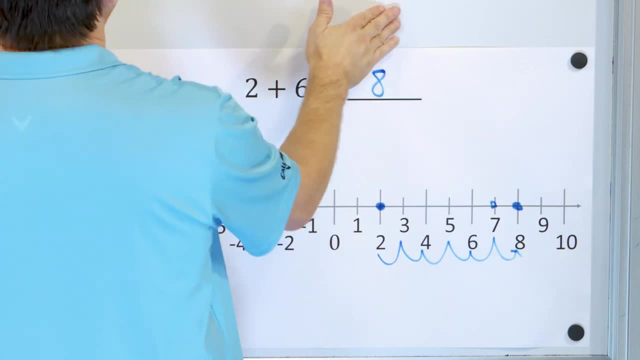 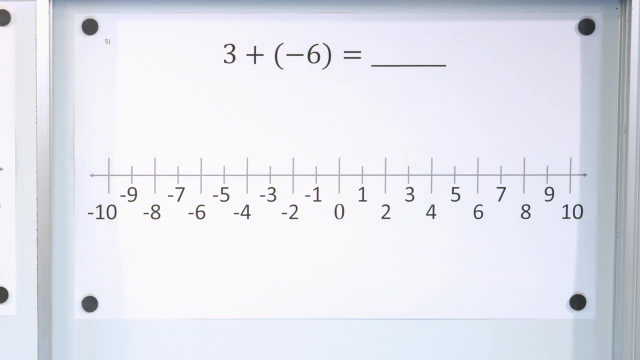 should be eight, And so two plus six is eight. Positive plus positive is positive, as we have said before. Now here we have a situation where we have a positive plus a negative. They're opposite signs. So the fast way to do it is just to say: OK, I'm adding something. 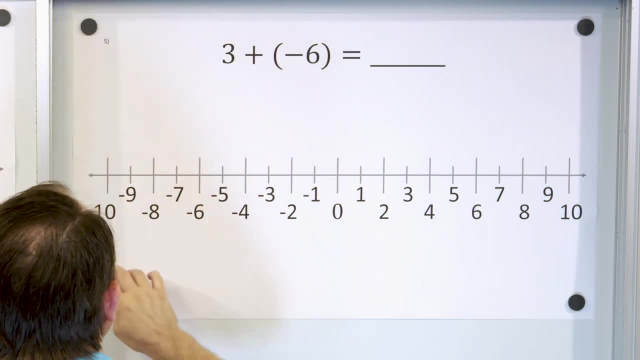 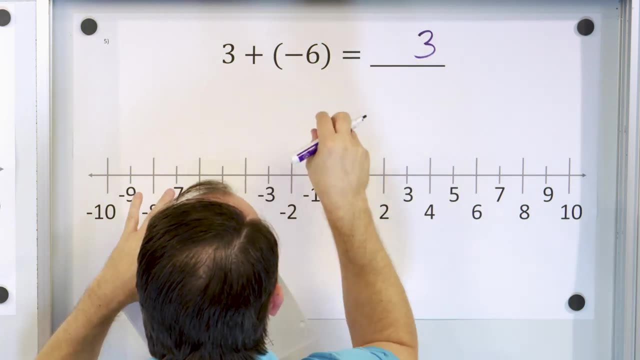 where I have positive, negative. They're different, different signs, So all I have to do is subtract Six minus three is three, And the sign of the answer just depends on which one of these is bigger in terms of absolute value. There's more debt here than money, So this one's the 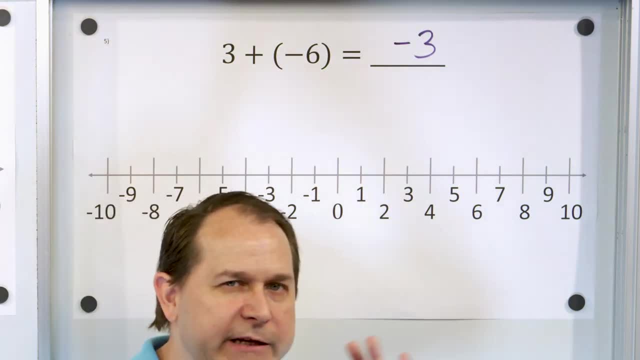 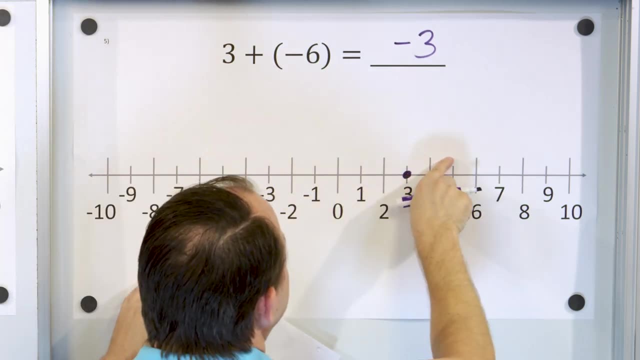 bigger absolute value. So the sign is negative. So without using any number line you can get the answer. Now, to use a number line, you start with three And usually when you add you go to the right, but you're adding debt. That means you move to the left. six units, One, two, three. Now I have 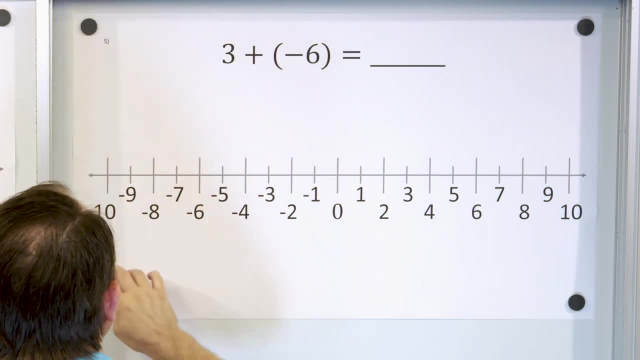 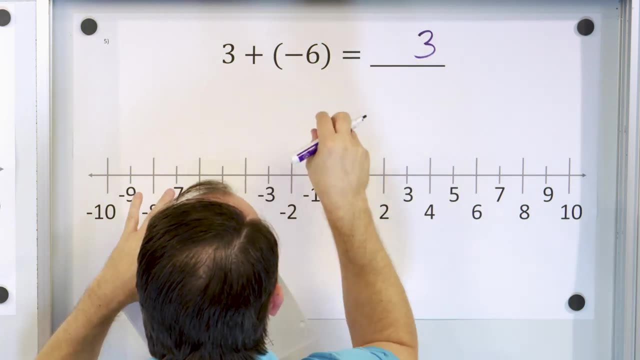 where I have positive, negative. They're different, different signs, So all I have to do is subtract Six minus three is three, And the sign of the answer just depends on which one of these is bigger in terms of absolute value. There's more debt here than money, So this one's the 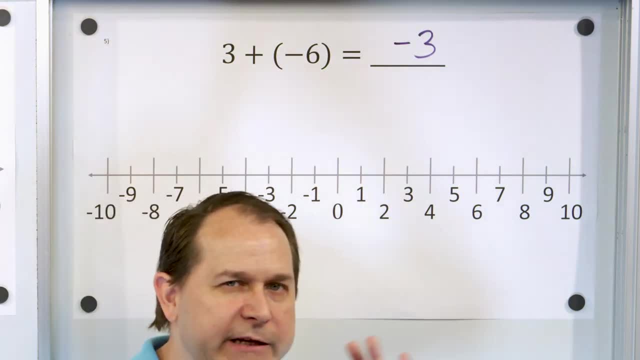 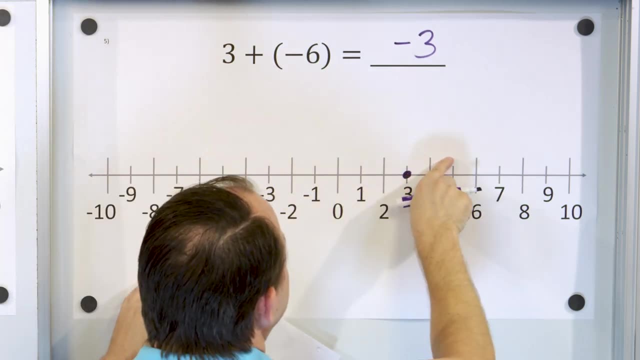 bigger absolute value. So the sign is negative. So without using any number line you can get the answer. Now, to use a number line, you start with three And usually when you add you go to the right, but you're adding debt. That means you move to the left. six units, One, two, three. Now I have 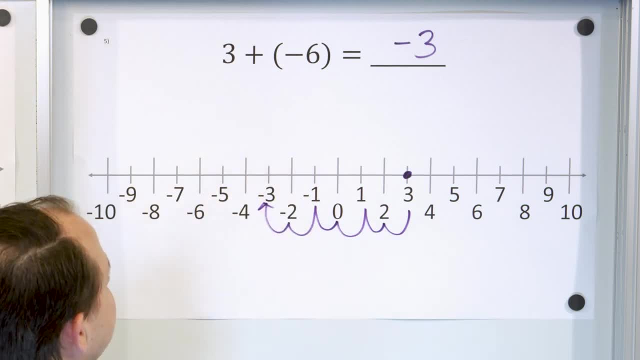 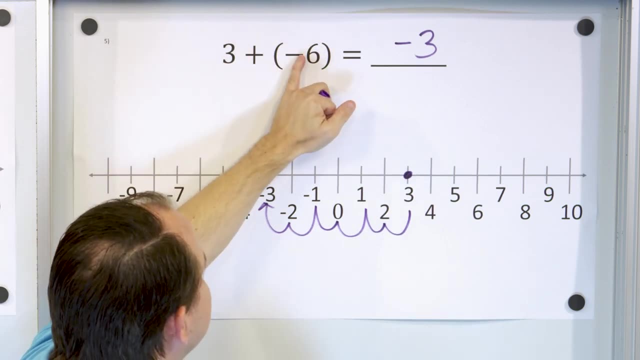 nothing. Four, five, six. Now I owe somebody three dollars, Because if I start with three dollars in my bank account and I borrow six dollars, then I'm going to use this to pay off three of the six dollars, But I'm still going to owe three dollars at the end. That's why the answer is negative. 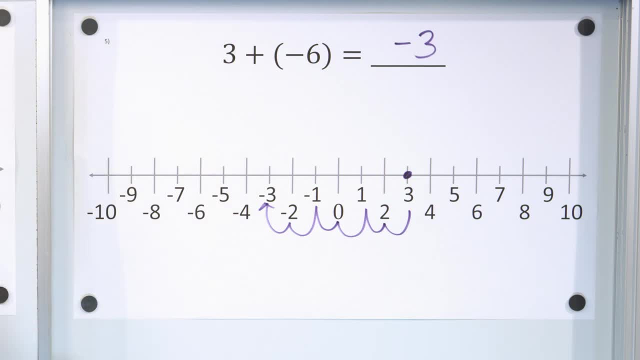 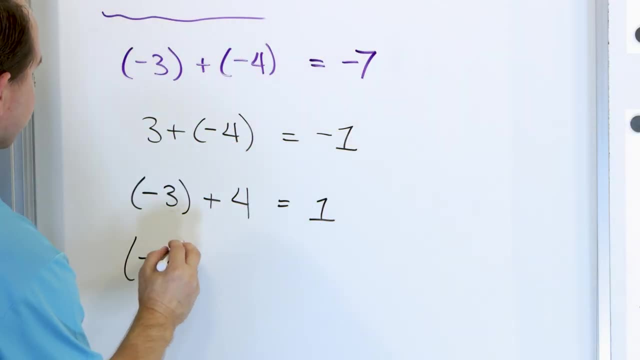 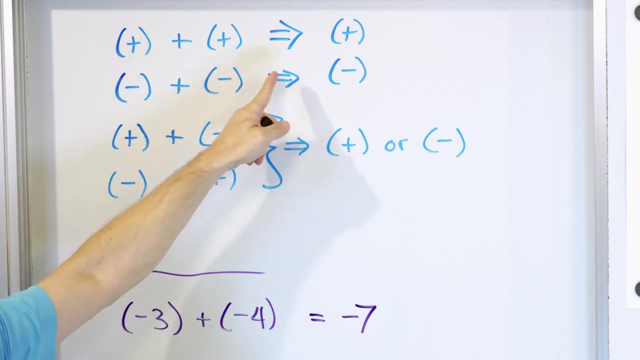 Three. Now, just for giggles, let's do a related problem, just to kind of get some practice with something else. What if it was negative three plus negative six. Right, We said positive plus positive, positive, negative plus negative, always negative. Here we have a negative plus. 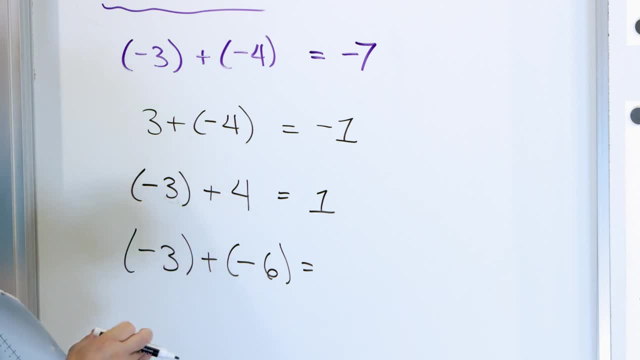 negative. So we know the answer has to be negative, But what is the answer going to be? Well, I start with owing someone three dollars and now I owe someone else six more dollars. So really, I'm in my mind, I'm adding: three plus six is nine, because that's the total debt and it. 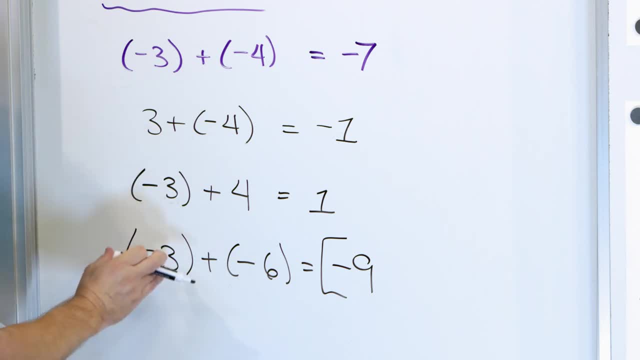 has to be negative. So it's going to be negative nine, because negative plus negative gives you negative, because debt plus more debt means I have to add the numbers and that's going to be the total debt that I have: Negative three plus a negative six, If you want to think about it on the number. 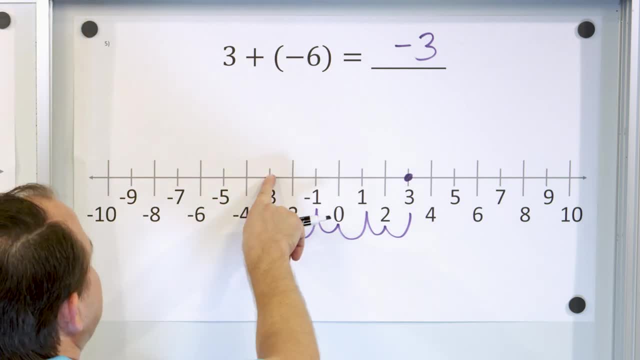 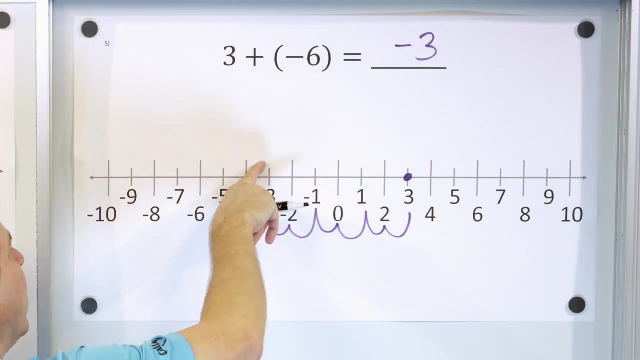 line negative three plus a negative six. If I started with negative three right here, this is where I would start and I take out more debt of six. I'm not going to take out more debt of six. I'm going to go to the right. I have to go to the left because I'm borrowing one, two, three, four. 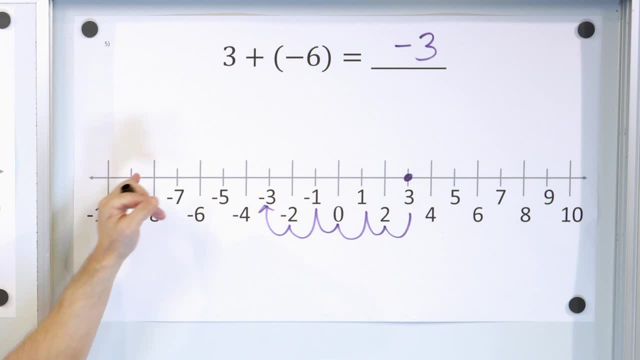 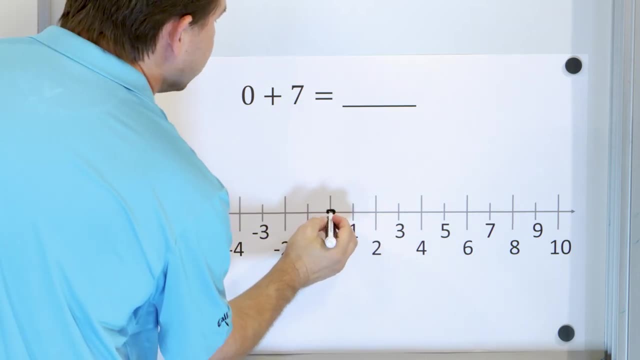 five, six, and I land on negative nine, which means I owe nine dollars, which is what I just wrote down. All right, Here's an easy problem. Zero plus seven means I start at zero and I move one, two, three, four, five, six, seven units to the right, And so, of course, the answer is seven. 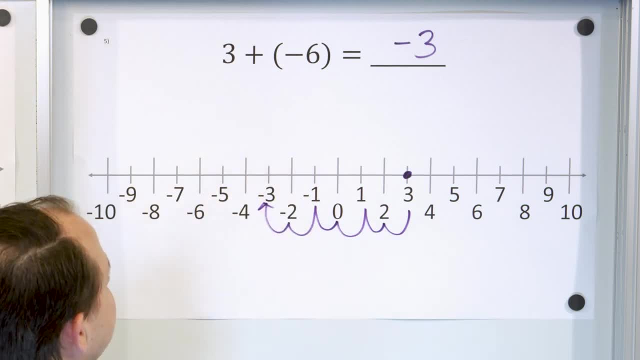 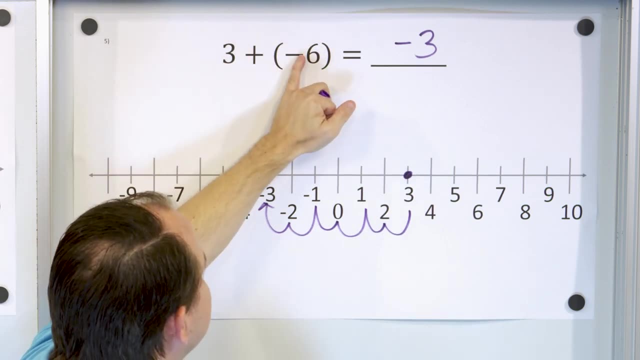 nothing. Four, five, six. Now I owe somebody three dollars, Because if I start with three dollars in my bank account and I borrow six dollars, then I'm going to use this to pay off three of the six dollars, But I'm still going to owe three dollars at the end. That's why the answer is negative. 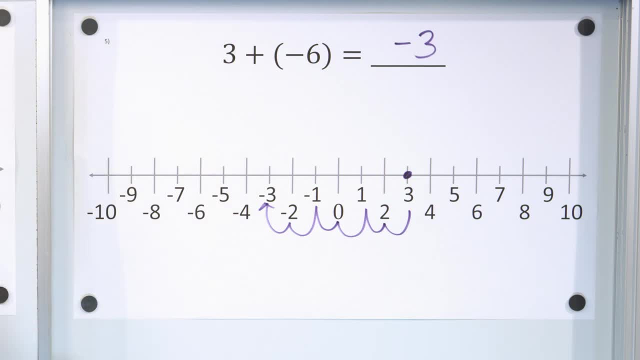 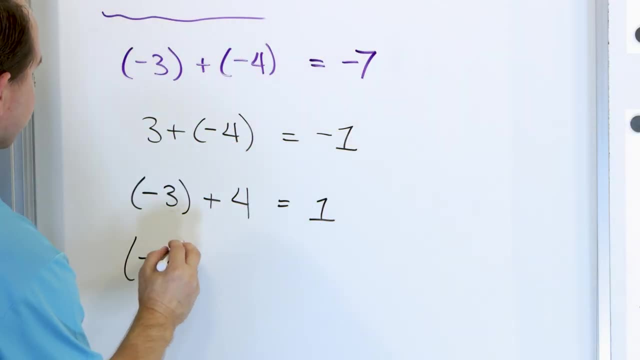 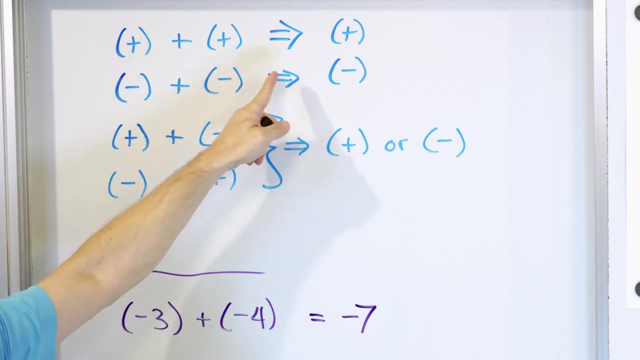 Three. Now, just for giggles, let's do a related problem, just to kind of get some practice with something else. What if it was negative three plus negative six. Right, We said positive plus positive, positive, negative plus negative, always negative. Here we have a negative plus. 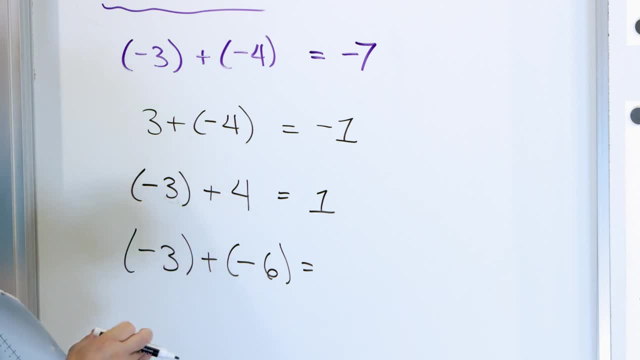 negative. So we know the answer has to be negative, But what is the answer going to be? Well, I start with owing someone three dollars and now I owe someone else six more dollars. So really, I'm in my mind, I'm adding: three plus six is nine, because that's the total debt and it. 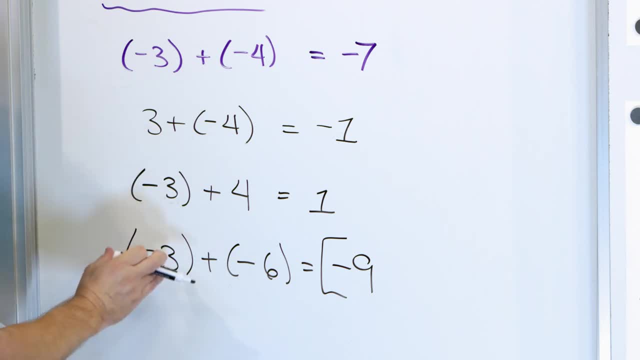 has to be negative. So it's going to be negative nine, because negative plus negative gives you negative, because debt plus more debt means I have to add the numbers and that's going to be the total debt that I have: Negative three plus a negative six, If you want to think about it on the number. 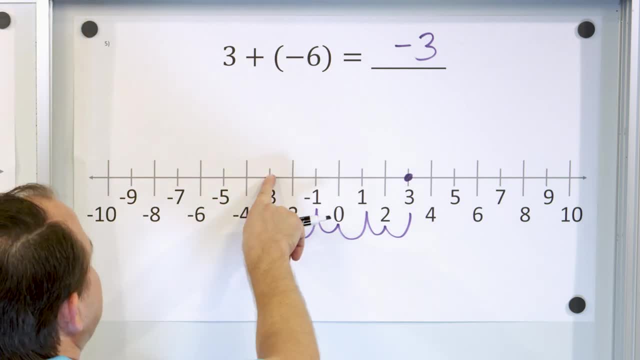 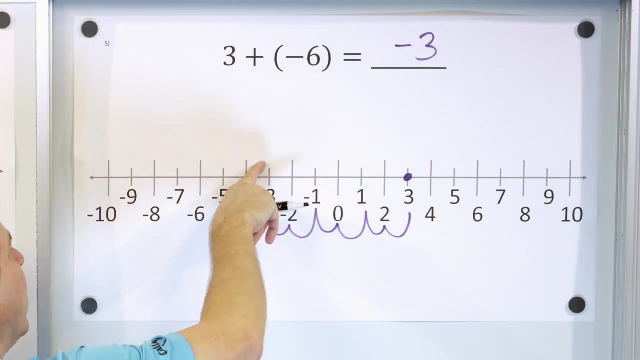 line negative three plus a negative six. If I started with negative three right here, this is where I would start and I take out more debt of six. I'm not going to take out more debt of six. I'm going to go to the right. I have to go to the left because I'm borrowing one, two, three, four. 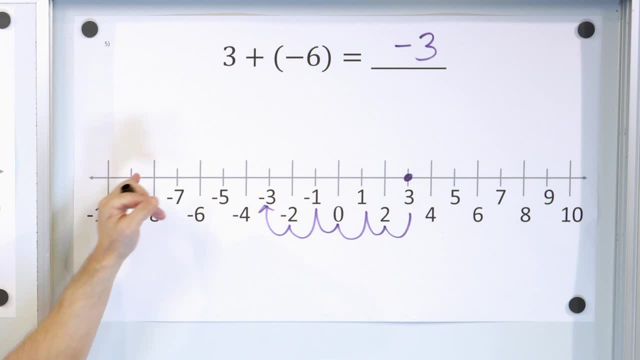 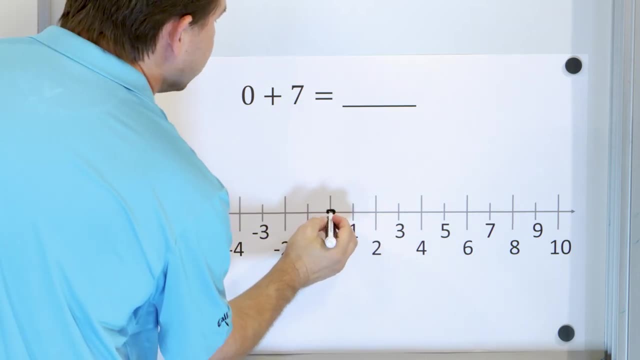 five, six, and I land on negative nine, which means I owe nine dollars, which is what I just wrote down. All right, Here's an easy problem. Zero plus seven means I start at zero and I move one, two, three, four, five, six, seven units to the right, And so, of course, the answer is seven. 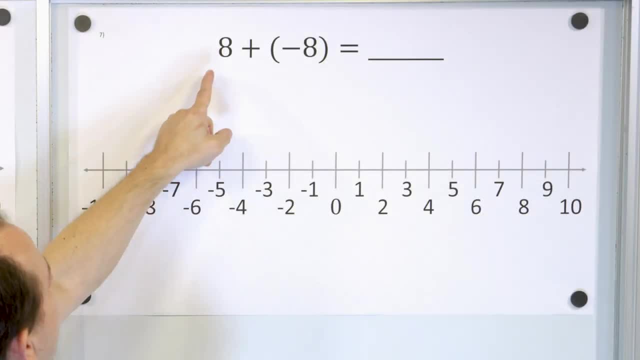 All right, Seven units, All right. Now here's an interesting problem. What if I start out with eight dollars? That's how much money I have, But then I borrow eight dollars. That means I take eight dollars of debt. How much is my actual worth now If I start with eight and I borrow? 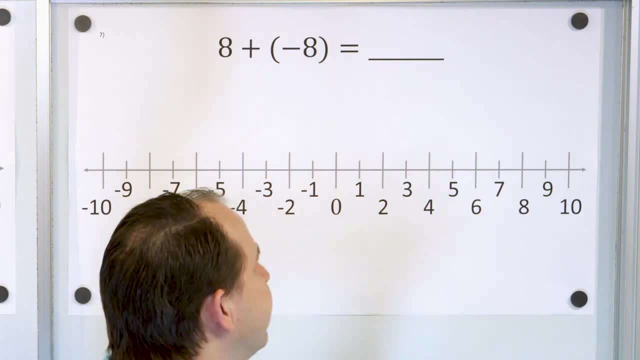 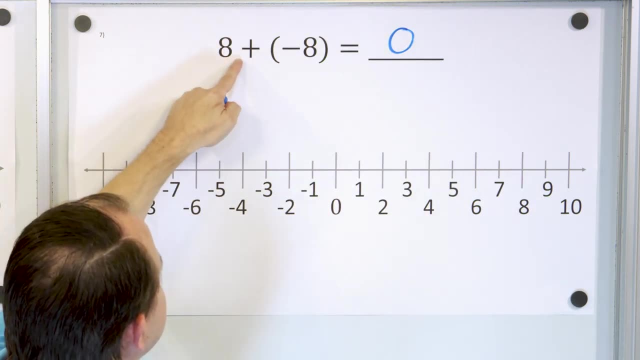 eight dollars. once I pay off the debt, I have nothing left, And so the answer to this- without really even looking at the at the chart here- is zero, And you can think about it that this is like the positive number is pulling, pulling you one way and the negative number is like pulling you. 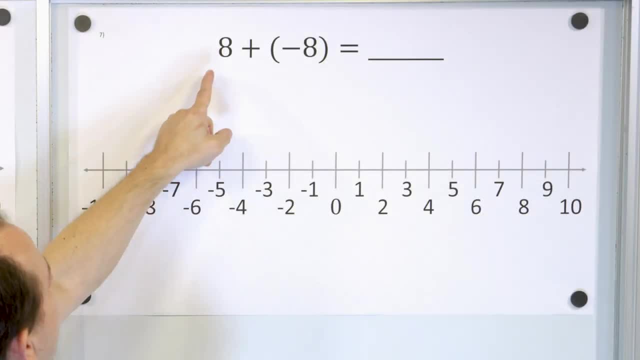 All right, Seven units, All right. Now here's an interesting problem. What if I start out with eight dollars? That's how much money I have, But then I borrow eight dollars. That means I take eight dollars of debt. How much is my actual worth now If I start with eight and I borrow? 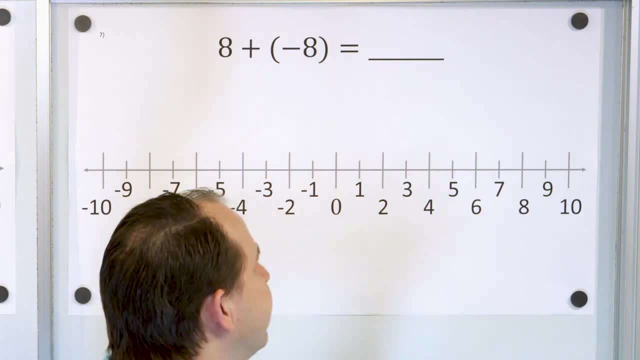 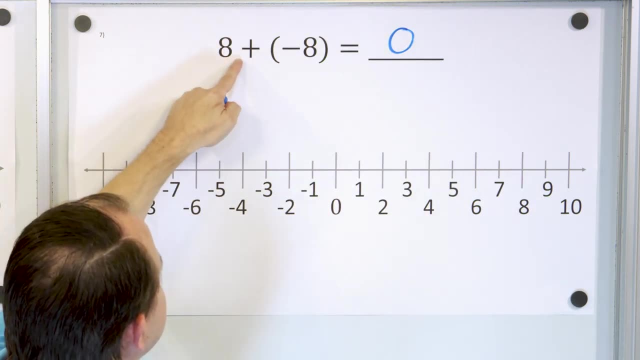 eight dollars. once I pay off the debt, I have nothing left, And so the answer to this- without really even looking at the at the chart here- is zero, And you can think about it that this is like the positive number is pulling, pulling you one way and the negative number is like pulling you. 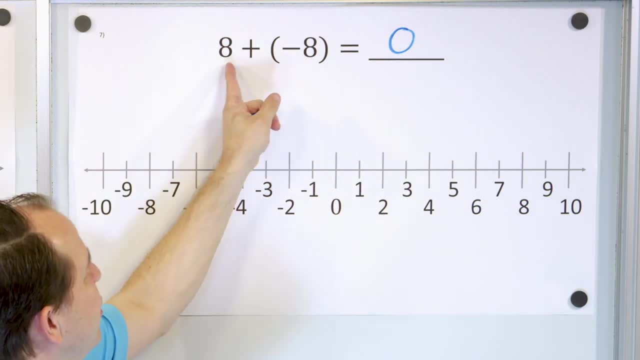 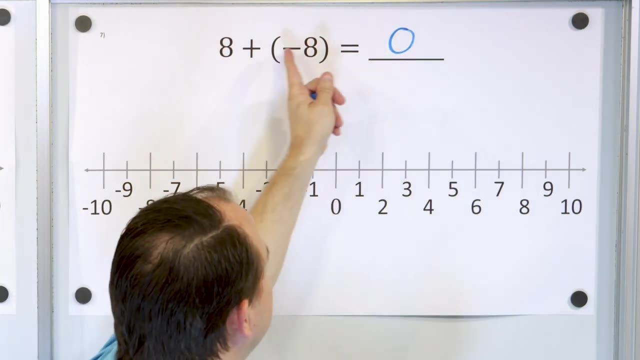 the other way And remember what I said whenever you add these. when you add two things that have opposite signs, you essentially subtract the numbers. Eight minus eight is zero And the sign goes with the bigger one, But both of them are the same size, So there is no sign on. 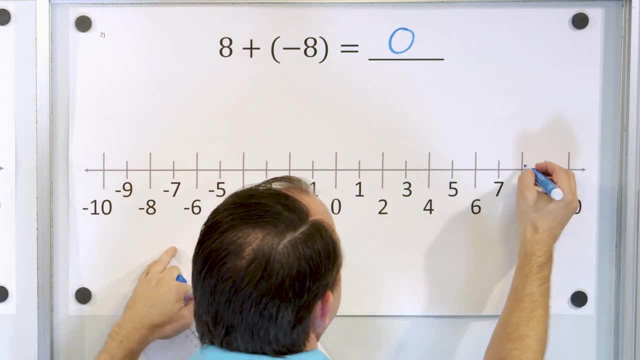 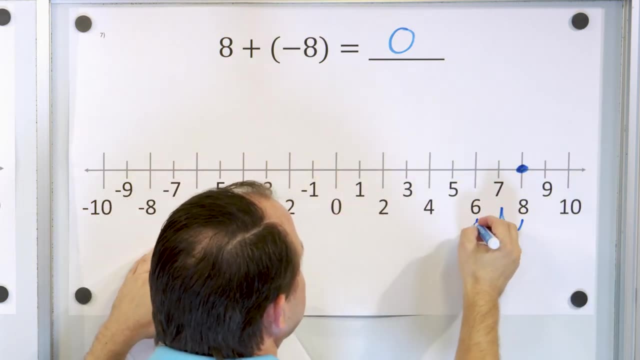 zero Right. So if you want to think about it in terms of a number line, you start with eight dollars right here and you add: But instead of going to the right, you're adding debt, which means you have to go to the left Eight units: three, four, five, six, seven and eight, And so. 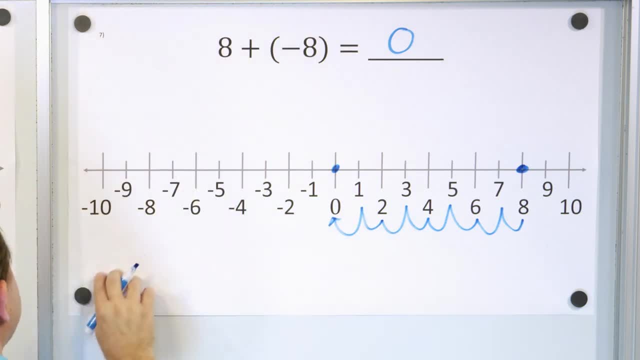 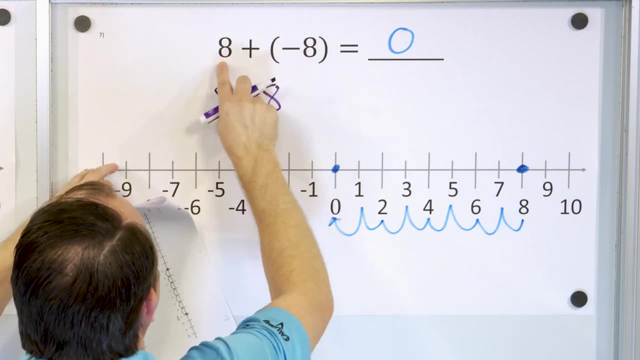 you land on the number zero. Now, if it helps you, you can also remember from the last lesson: anytime we add the opposite sign, we can treat it as subtraction. So eight plus a negative eight is the same as eight minus eight, which you already know to be. 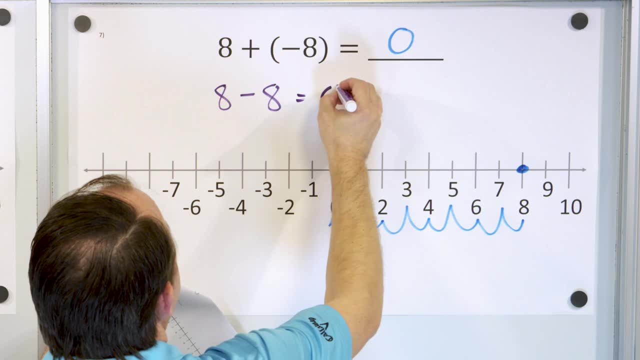 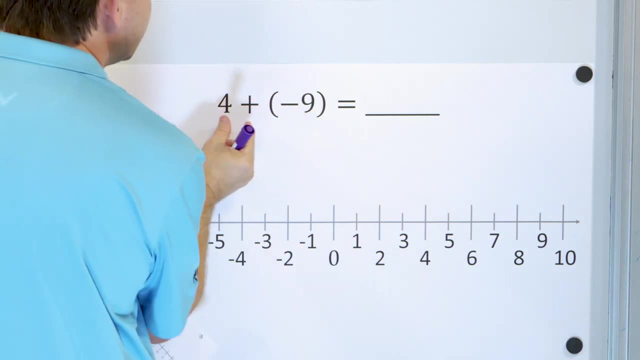 zero. So it's the same exact thing. All right. Whatever way you want to think about is fine with me, All right. Next problem: Let's take a look at four plus a negative nine. You have a positive amount of money you have pulling one way and you have a nine dollars of debt pulling you the other. 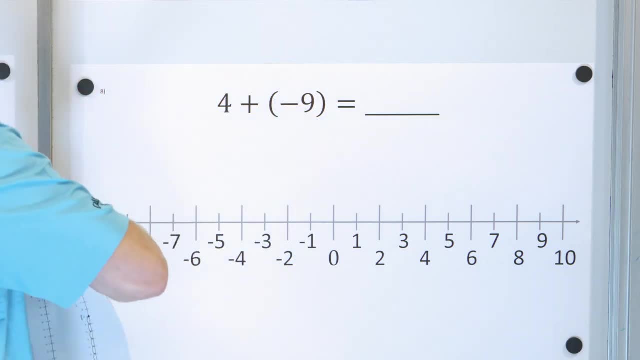 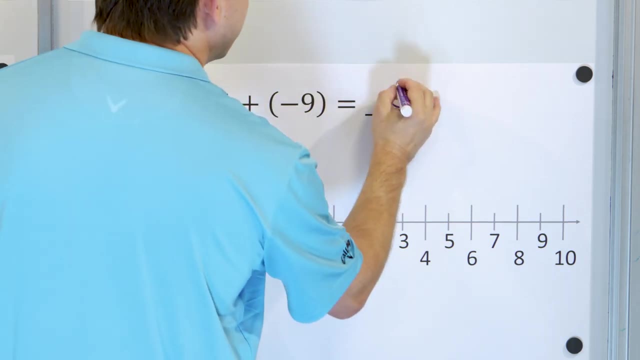 way Which one's going to win. I have more debt, So that one is the bigger number. The answer will be negative. To get the number, you just take nine minus four. They're opposite signs. Nine minus four is five. This is the bigger absolute value. So the answer is negative: five Now. 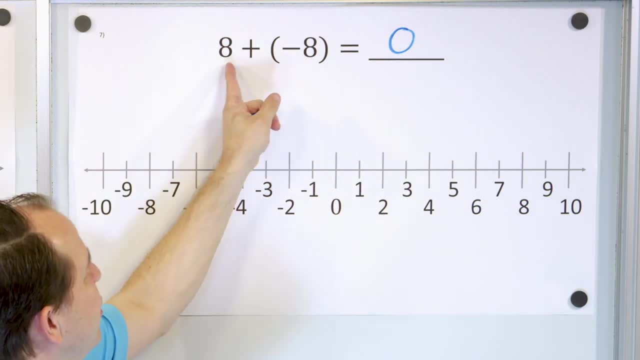 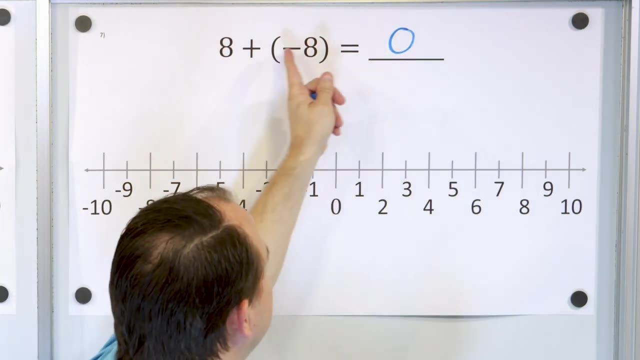 the other way And remember what I said whenever you add these. when you add two things that have opposite signs, you essentially subtract the numbers. Eight minus eight is zero And the sign goes with the bigger one, But both of them are the same size, So there is no sign on. 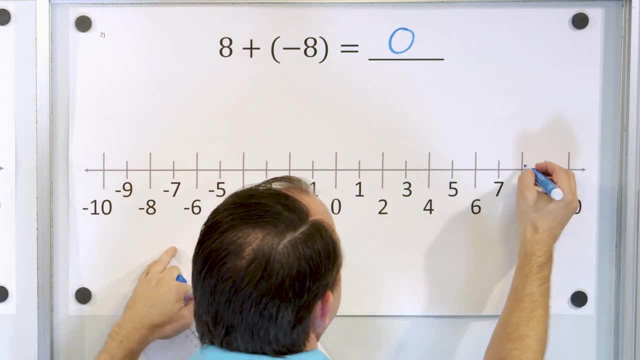 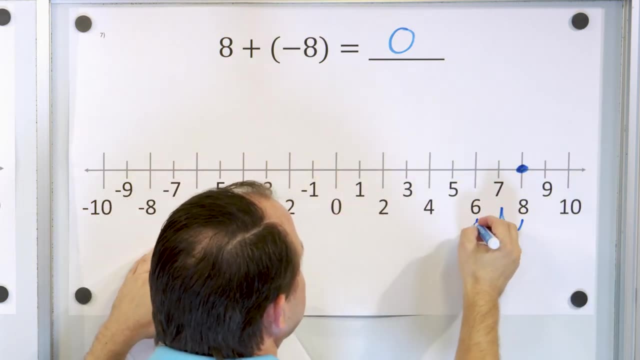 zero Right. So if you want to think about it in terms of a number line, you start with eight dollars right here and you add: But instead of going to the right, you're adding debt, which means you have to go to the left Eight units: three, four, five, six, seven and eight, And so. 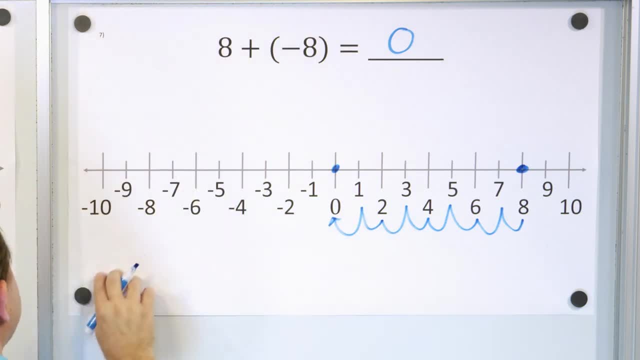 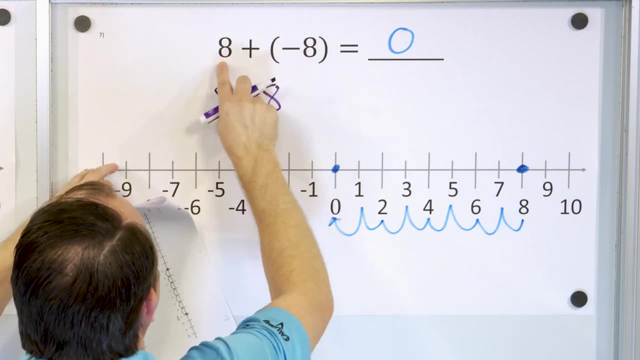 you land on the number zero. Now, if it helps you, you can also remember from the last lesson: anytime we add the opposite sign, we can treat it as subtraction. So eight plus a negative eight is the same as eight minus eight, which you already know to be. 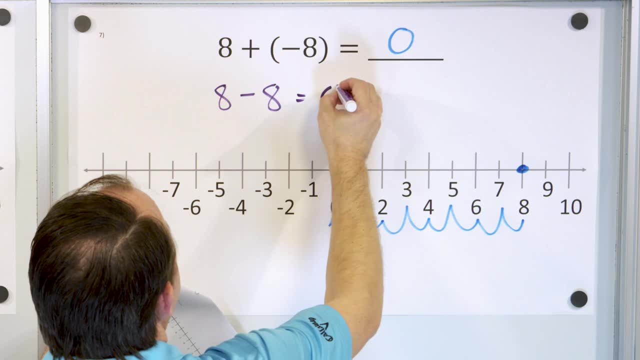 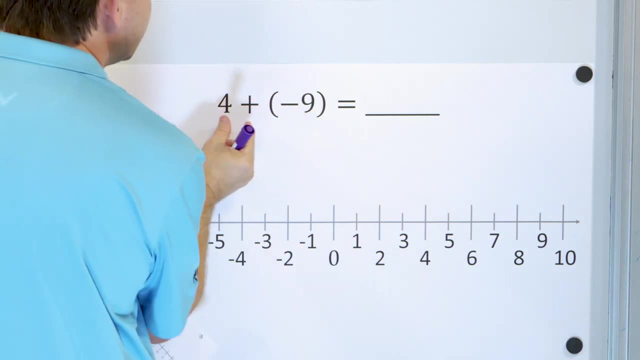 zero. So it's the same exact thing. All right. Whatever way you want to think about is fine with me, All right. Next problem: Let's take a look at four plus a negative nine. You have a positive amount of money you have pulling one way and you have a nine dollars of debt pulling you the other. 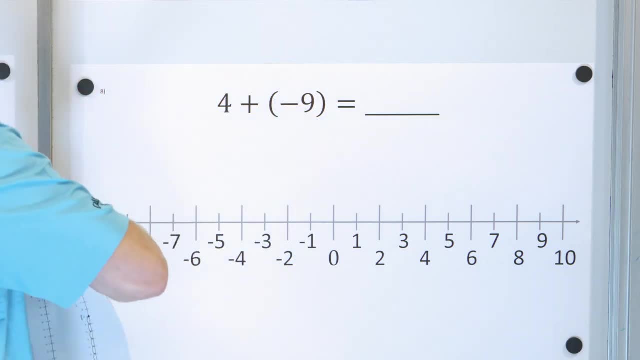 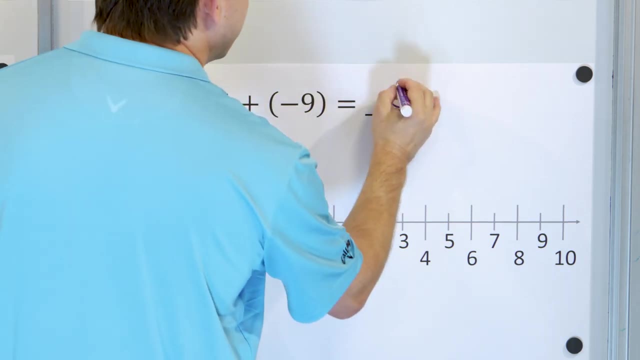 way Which one's going to win. I have more debt, So that one is the bigger number. The answer will be negative. To get the number, you just take nine minus four. They're opposite signs. Nine minus four is five. This is the bigger absolute value. So the answer is negative: five Now. 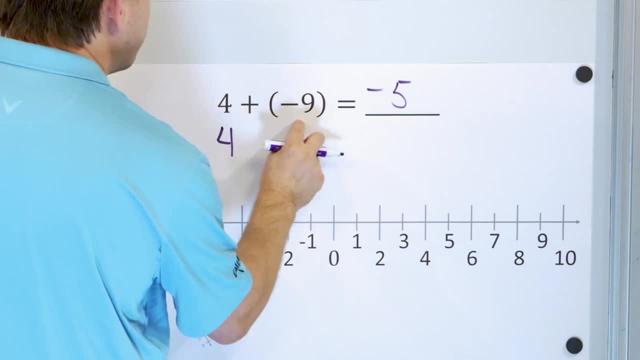 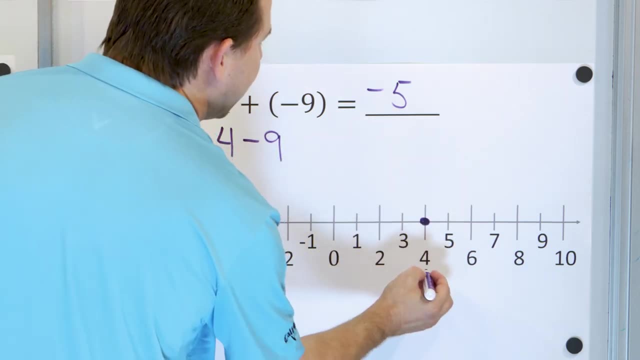 if you want to think about it in terms of subtraction, you can write this as four minus nine, which means starting with four dollars and subtracting nine away. If I start with four dollars and go down by nine, one, two, three, four, five, six, seven, eight and nine, I land. 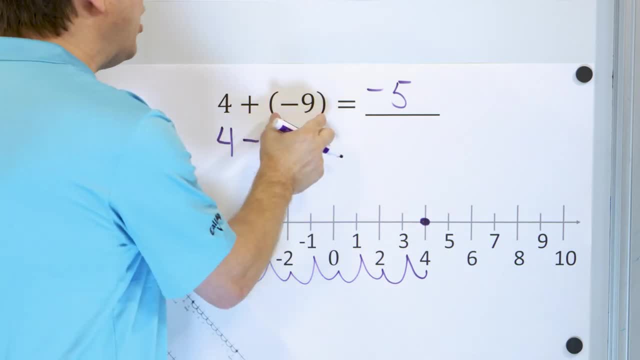 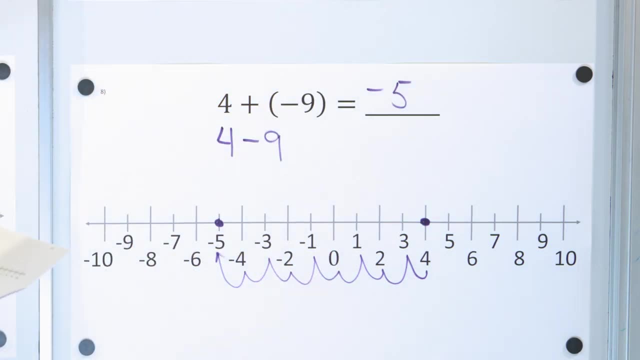 on negative five. So if I really do start with four dollars and then I borrow nine dollars, then once I pay back part of the debt, I'm still going to owe five dollars. That's why you land on a negative number, negative five like that. All right, The sign of this goes with the. 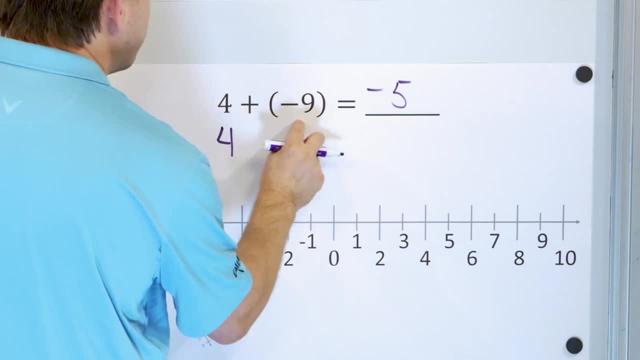 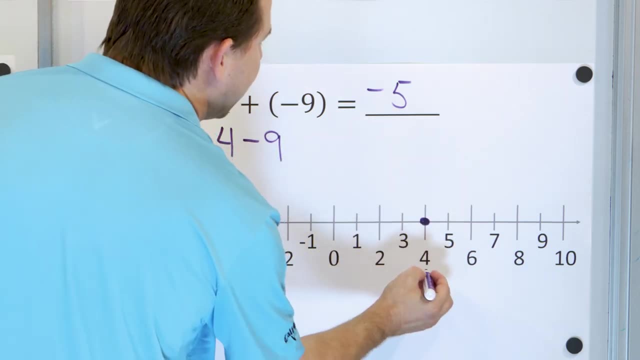 if you want to think about it in terms of subtraction, you can write this as four minus nine, which means starting with four dollars and subtracting nine away. If I start with four dollars and go down by nine, one, two, three, four, five, six, seven, eight and nine, I land. 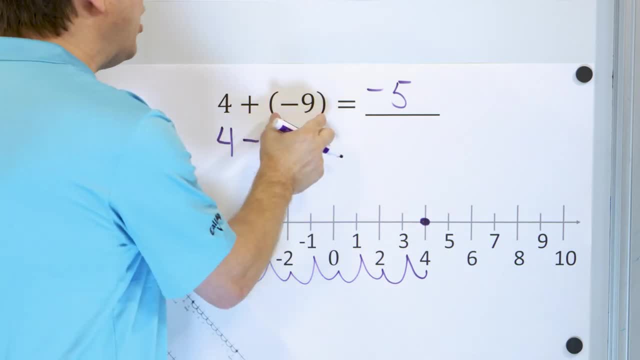 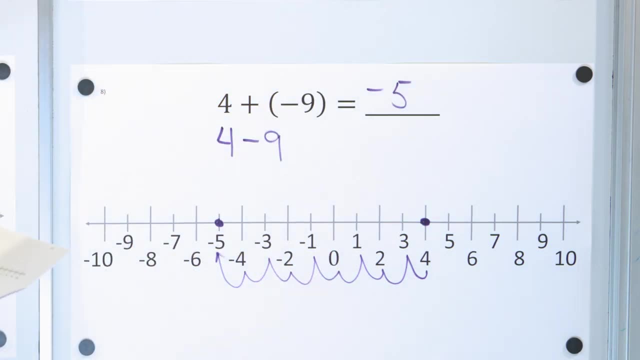 on negative five. So if I really do start with four dollars and then I borrow nine dollars, then once I pay back part of the debt, I'm still going to owe five dollars. That's why you land on a negative number, negative five like that. All right, The sign of this goes with the. 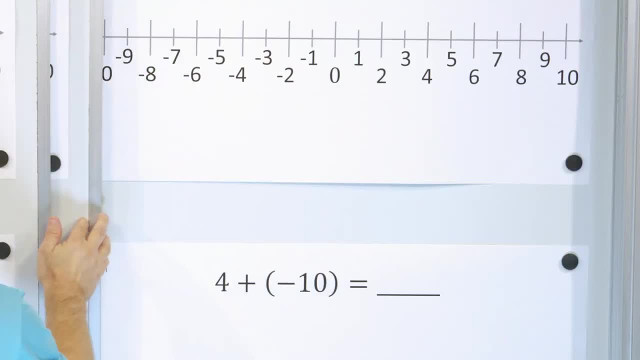 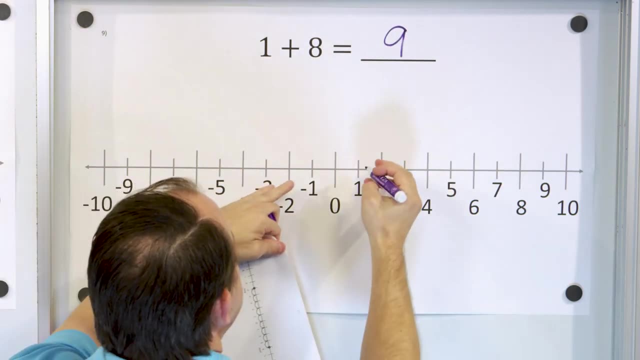 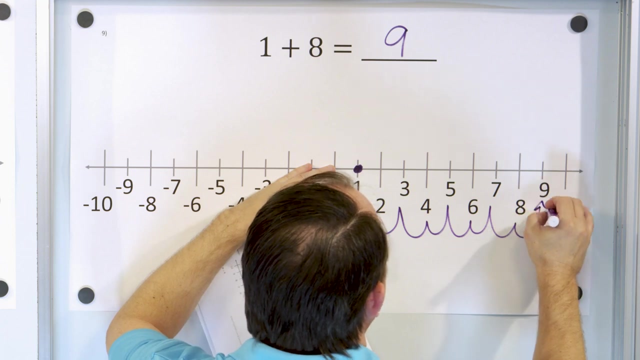 bigger of the absolute values, All right. Problem number nine: one plus eight. Positive plus positive always gives you a positive number If you start with one and you go eight units to the right: one, two, three, four, five, six, seven, eight, And there you go, You land on nine. 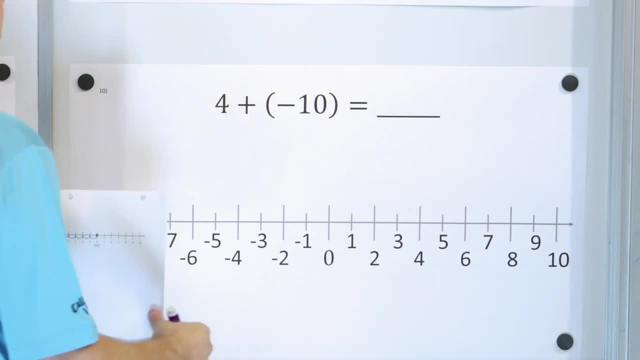 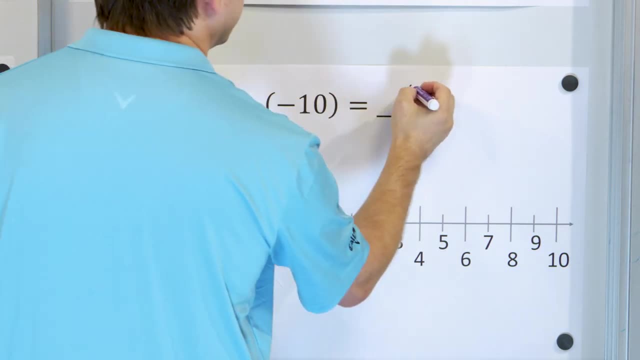 All right, Here's our very last problem. Four plus a negative ten, You have opposite signs, right? Just as we said. So when you have opposite signs and you're adding them, you just subtract the numbers. Ten minus four is six, And the sign of it goes with the bigger. 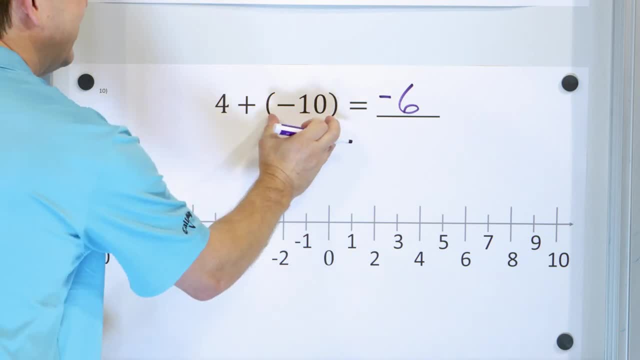 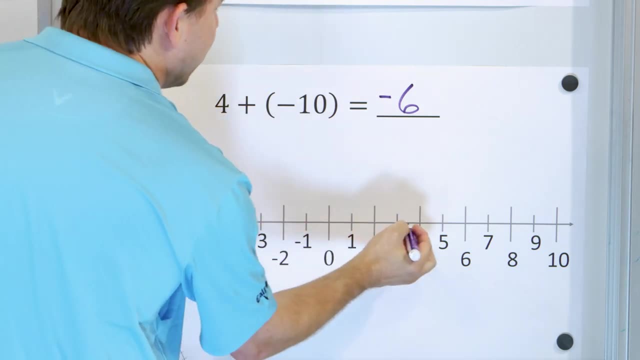 absolute value. In this case, negative, because this is the bigger The debt is bigger than the money you have, And so once you subtract them, the answer is a debt there. So if you were to start with four dollars in your bank account and add to it ten dollars of debt, you would not go. 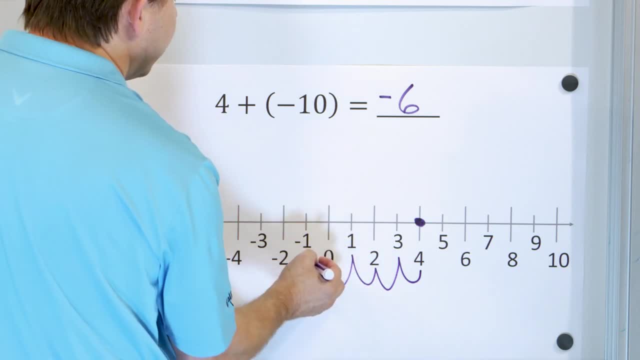 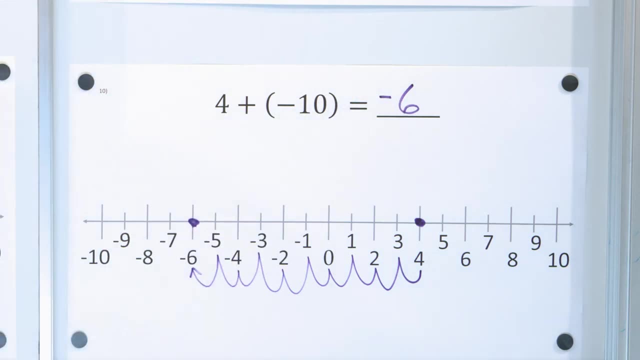 to the right. You would go to the left One, two, three, four, five, six, seven, eight, nine, ten And you would land on negative six. And that means you would have six dollars of debt left over. And if it helps you any time, we are adding the opposite like this. we said we can treat it as 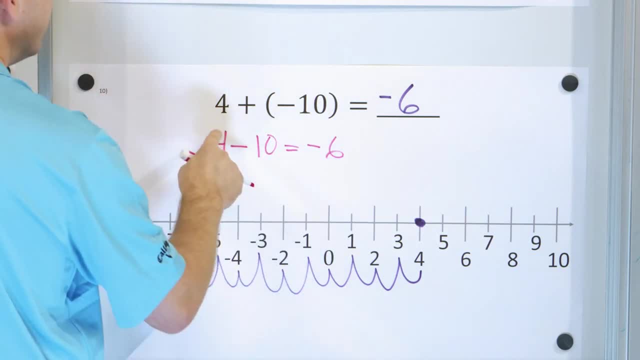 subtraction. And this is exactly the same exact thing. Four minus ten is also negative six. for the same reason, because if I start at four dollars and I subtract ten, I'm going to go down ten units. I'm going to land on negative six, just like this. So here we have started the 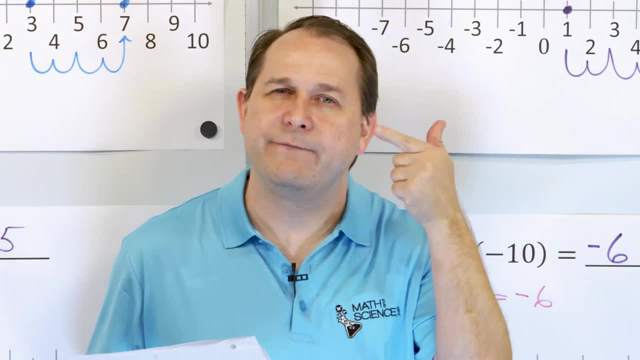 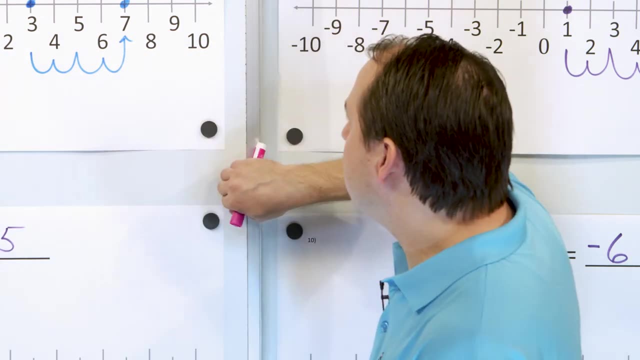 process of adding integers. It takes a little while for it to fully bake In your head, All right, And so I want you to watch this and solve all of these problems yourself. The bottom line is: we have these rules, but ultimately, you're not going to have to memorize. 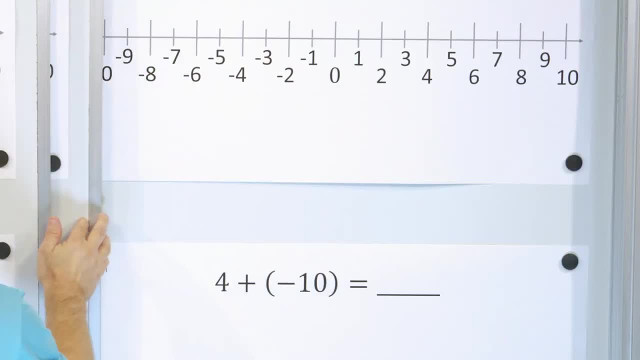 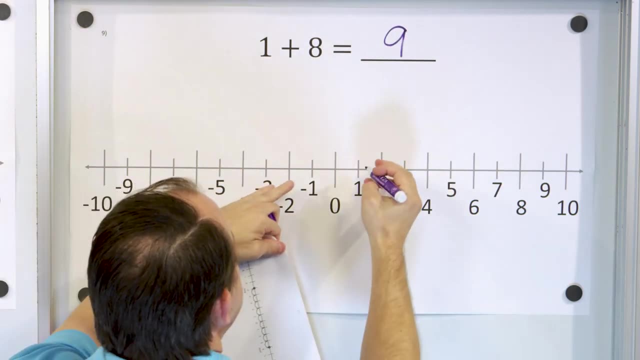 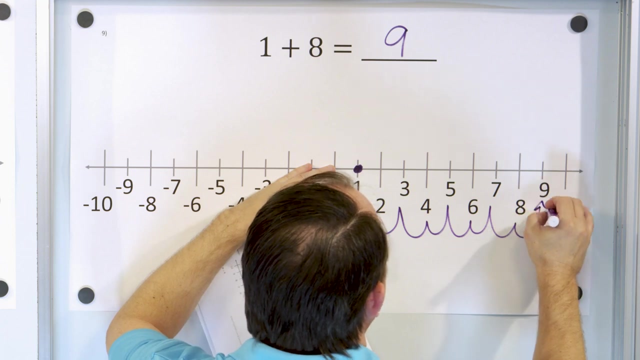 bigger of the absolute values, All right. Problem number nine: one plus eight. Positive plus positive always gives you a positive number If you start with one and you go eight units to the right: one, two, three, four, five, six, seven, eight, And there you go, You land on nine. 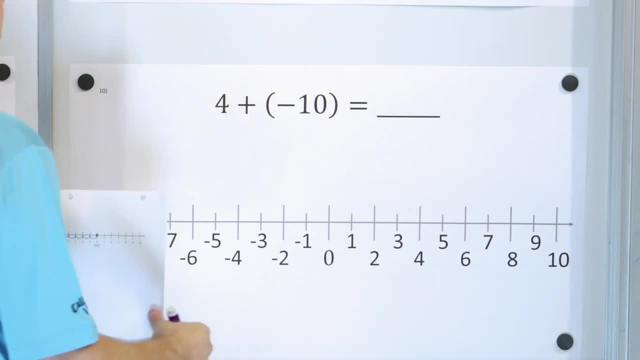 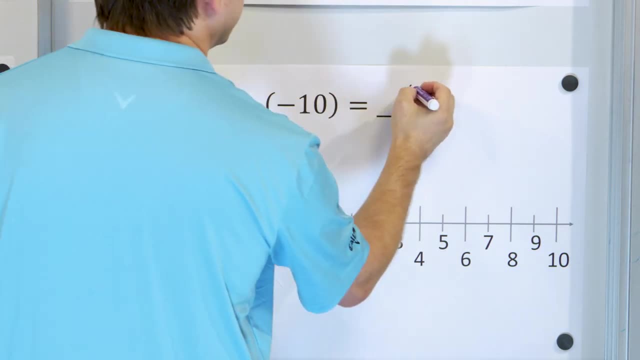 All right, Here's our very last problem. Four plus a negative ten, You have opposite signs, right? Just as we said. So when you have opposite signs and you're adding them, you just subtract the numbers. Ten minus four is six, And the sign of it goes with the bigger. 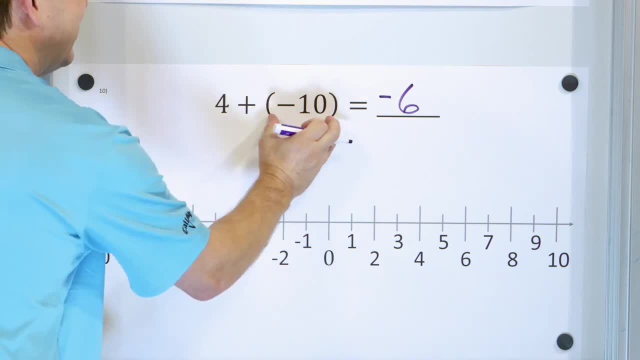 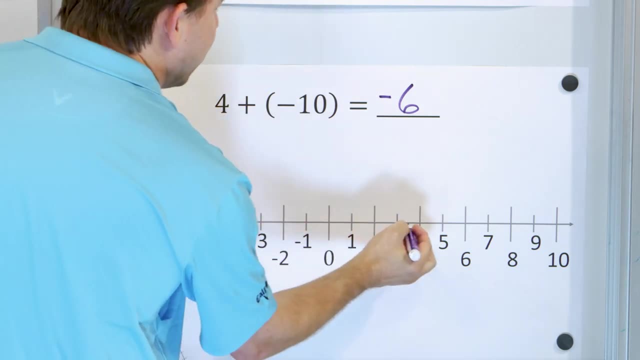 absolute value. In this case, negative, because this is the bigger the debt is bigger than the money you have, And so once you subtract them, the answer is a debt there. So if you were to start with four dollars in your bank account and add to it ten dollars of debt, you would not go to. 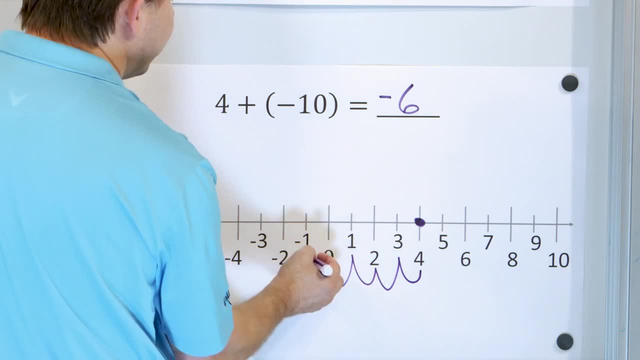 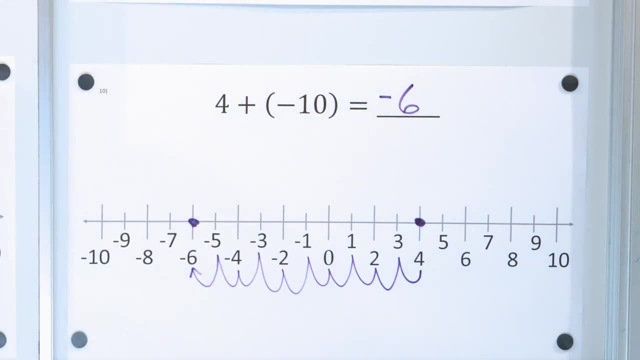 the right, You will go to the left One, two, three, four, five, six, seven, eight, nine, ten And you would land on negative six. That means you would have six dollars of debt left over And if it helps you, anytime we have, we are adding the opposite like this: we said we: 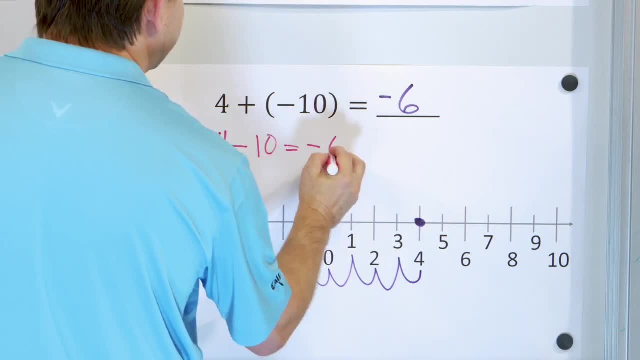 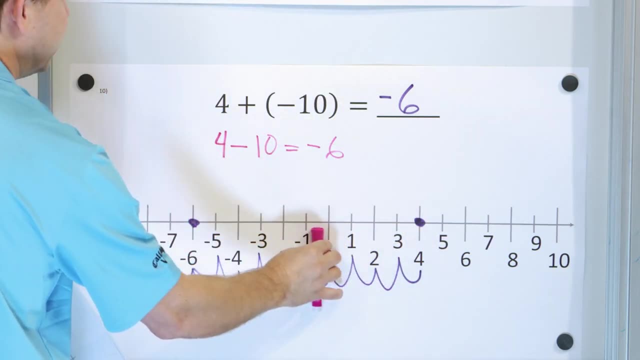 can treat it as subtraction, And this is exactly the same exact thing. Four minus ten is also negative six. for the same reason, because if I start at four dollars and I subtract ten, I'm going to go down ten units. I'm going to land on negative six, just like this. 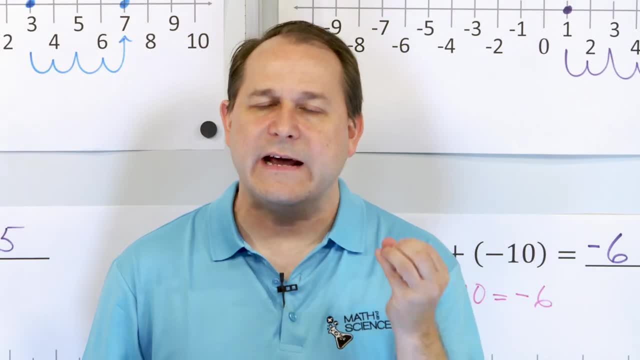 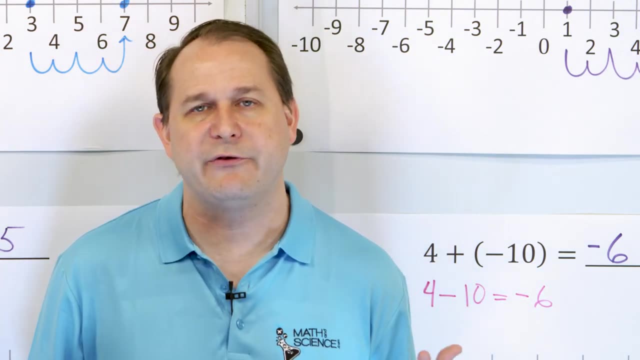 So here we have started the process of adding integers. It takes a little while for it to fully in your head, All right, And so I want you to watch this and solve all of these problems yourself. The bottom line is: we have these rules, but ultimately, you're not going to have to memorize. 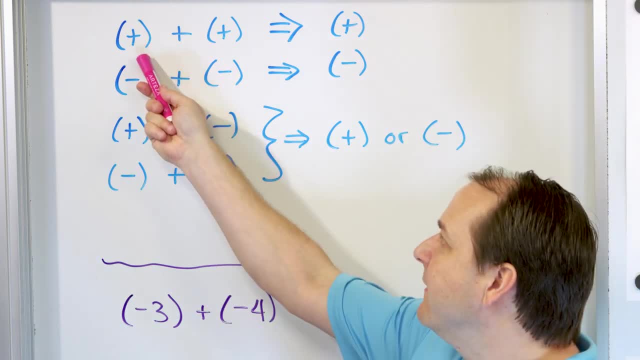 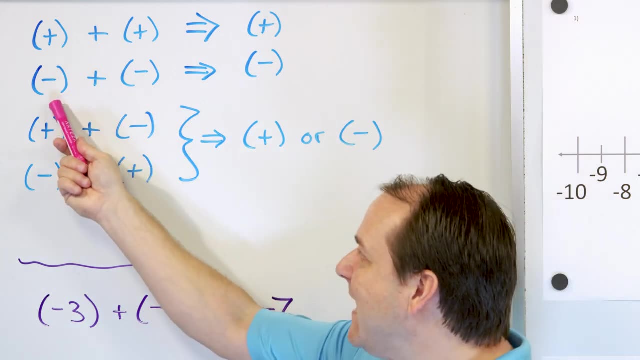 them because you're just going to remember them after a while. When you have positive numbers plus positive numbers, you're always going to get a positive answer. That's like regular arithmetic from third grade. If you have debt negative plus more debt negative, then the answer will always. 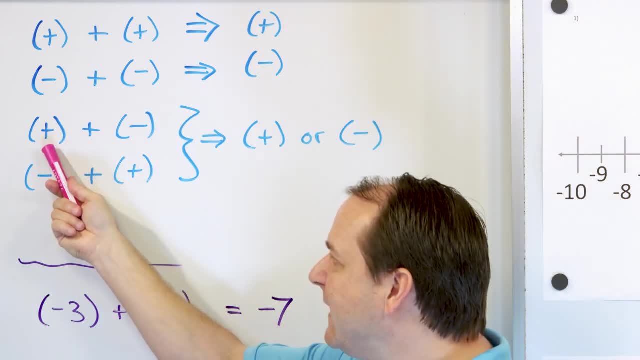 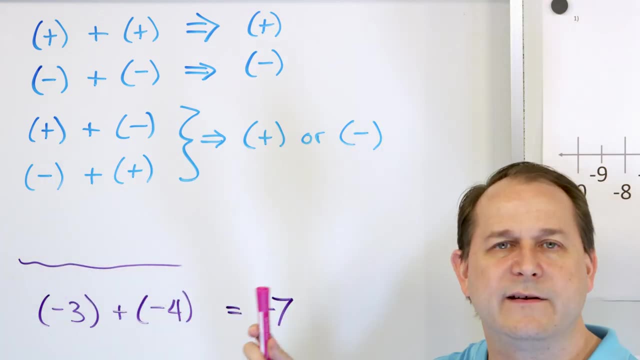 be more debt, which is negative. But if you have some actual money and you take on some debt, or if you start with some debt and take on some money, then the answer can be either one of positive or negative sign, And which one will win is going to depend on which one of